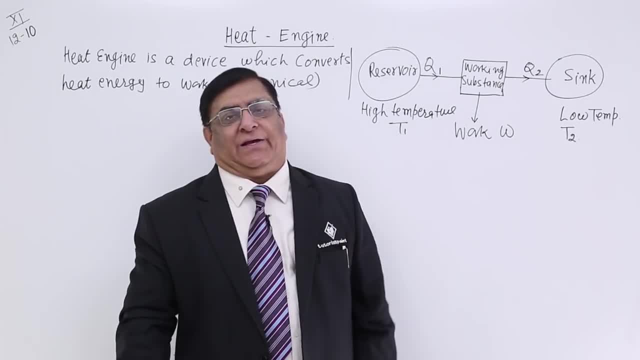 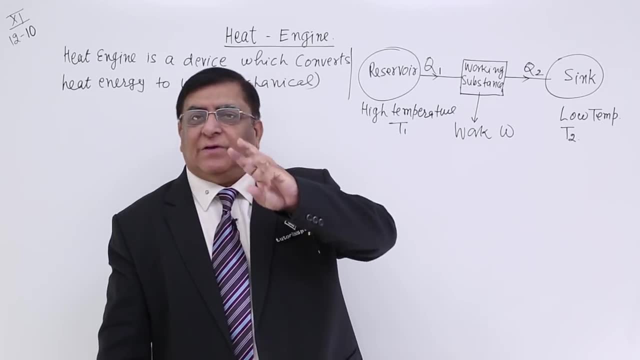 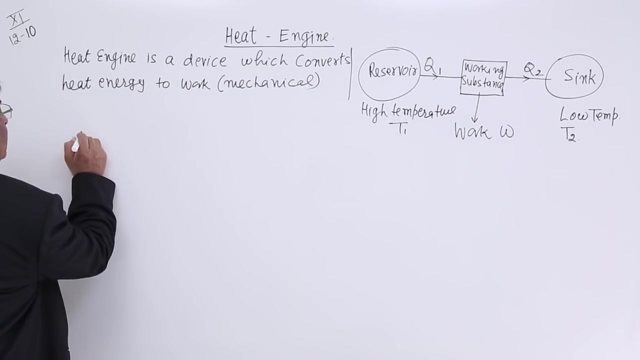 So that is conversion. So that is conversion of heat energy to mechanical energy. Now, with reference to physics, we divide it into three parts. Heat engine is divided into three main parts. One is we call it reservoir of heat. From there we will take heat energy. Reservoir of heat. 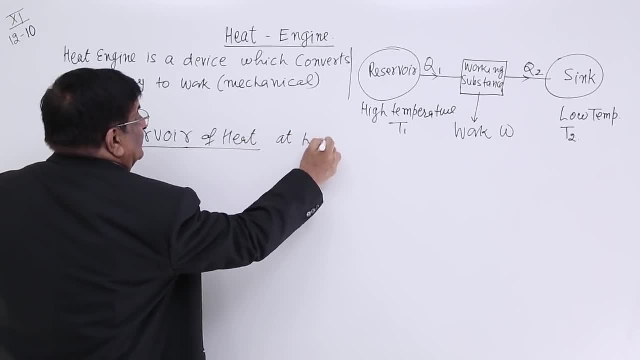 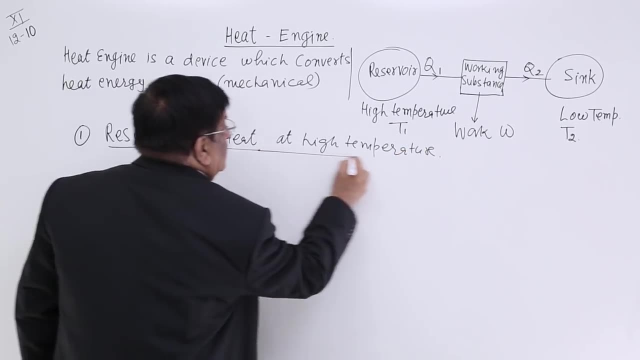 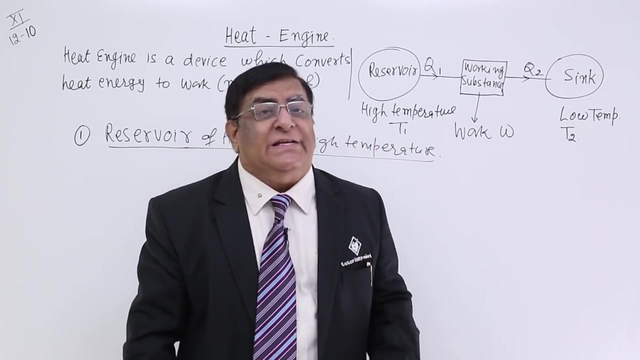 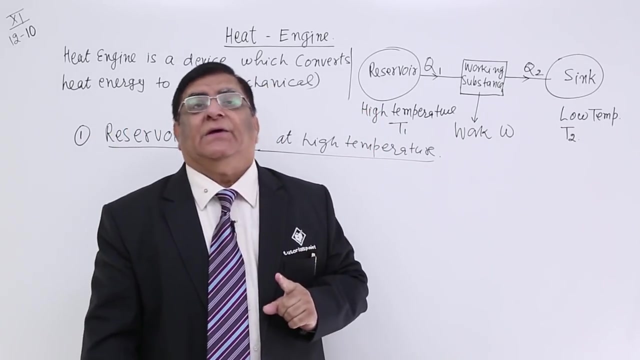 And it is a device. It is at high temperature. At high temperature, When we burn petrol in our engine, that mixture becomes the reservoir. What is specially of the reservoir? in physics, The specialty of the reservoir is that you can take any amount of heat from it and whatever amount you heat, you take from it. 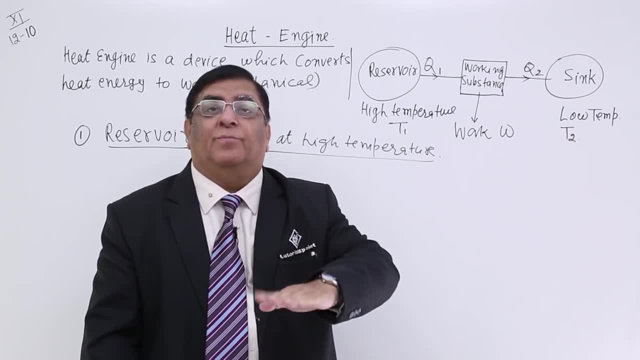 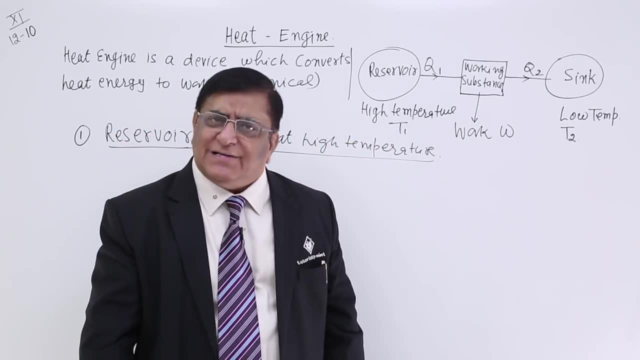 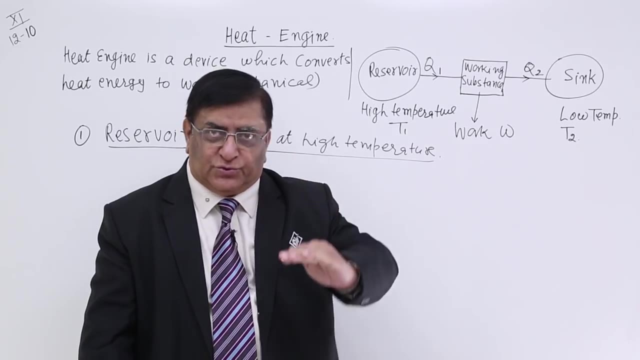 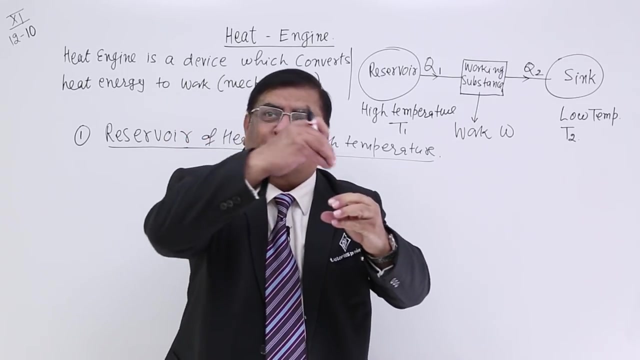 Its temperature will not become lower. Its temperature will remain same hot. Does it happen? Yes, it does happen, Because when we burn the petrol, the temperature is 400 degree. We use it, move our car, convert it to mechanical energy, Again we burn the next drop of the petrol, That is, again bring it to 400. Again, we burn the petrol. 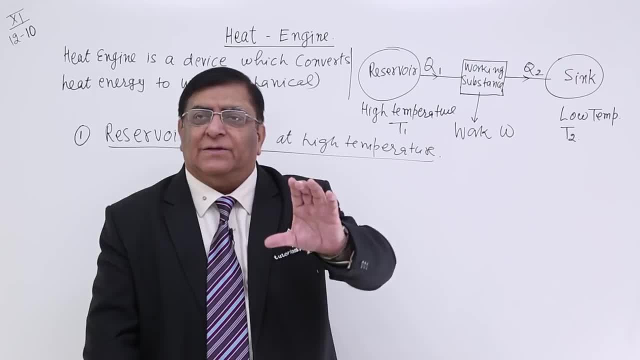 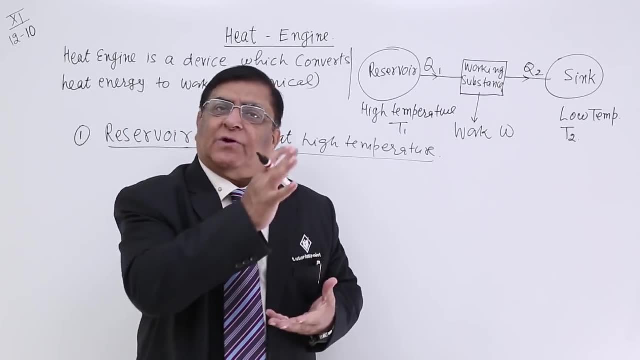 Again we burn the petrol. Again bring it to 400.. So every time The burning petrol contains that is our reservoir And it is temperature remained 400. And whatever amount of heat we need, we keep running the car. We have the stock of petrol. 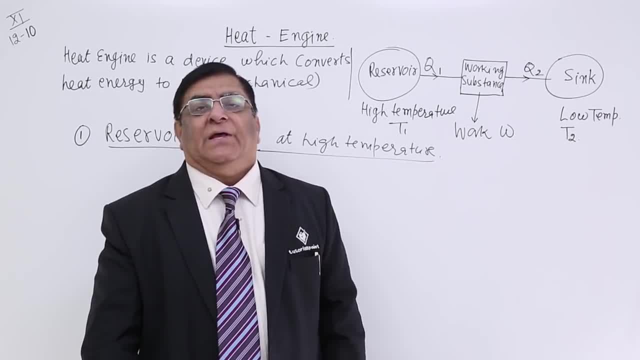 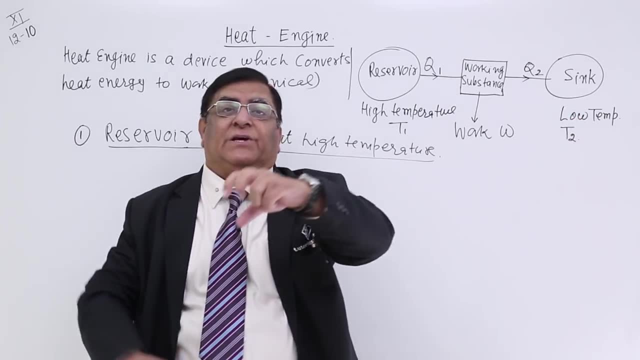 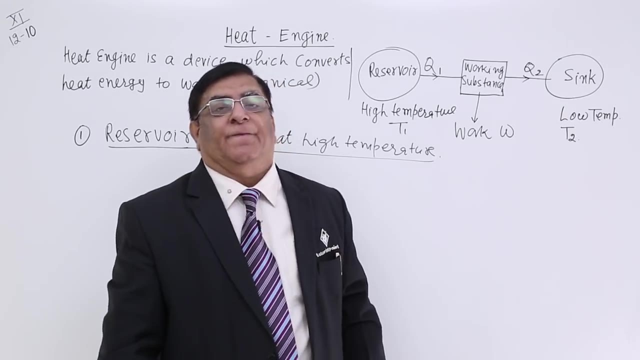 So this is the definition of reservoir. Another example you can say in terms of water: We have a sea of water And you take out any amount of water from the sea. its level does not go down. that is a reservoir. so we assume that in our heat engine we have 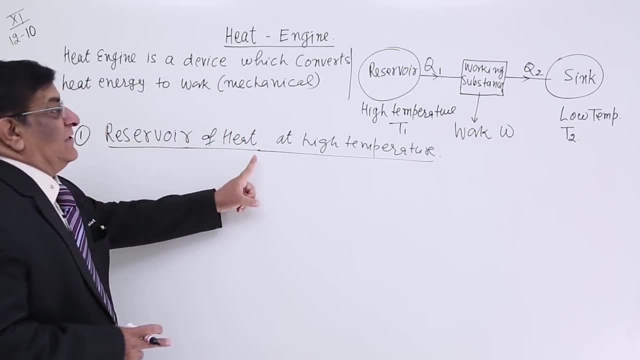 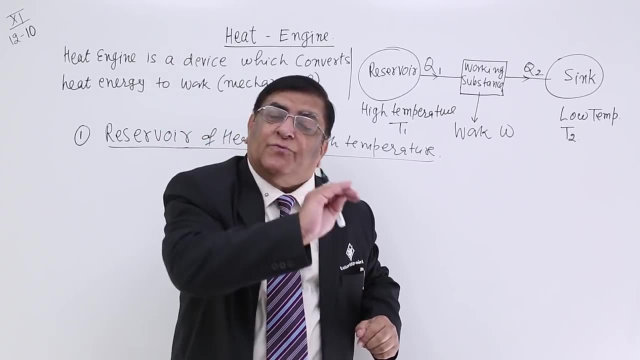 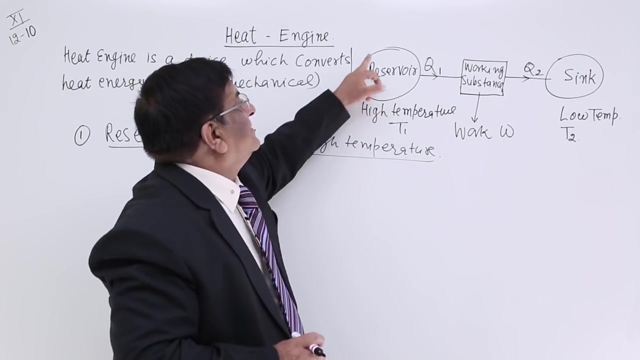 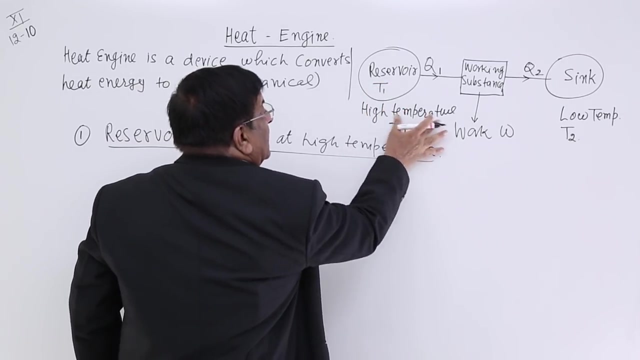 one source of energy and that is a heat reservoir at high temperature, because the high temperature will facilitate the flow of energy to a lower temperature. so it should be at a high temperature. and here is schematic diagram of a reservoir. this has a very high temperature, t1. okay, 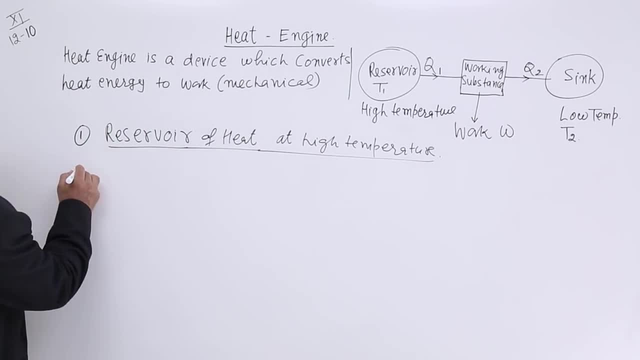 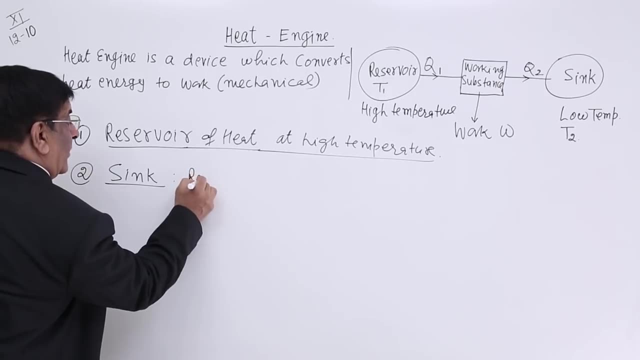 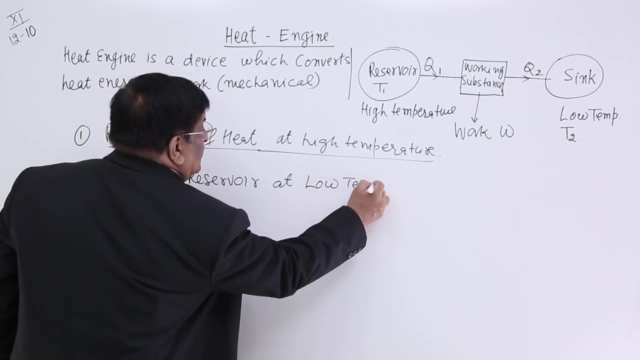 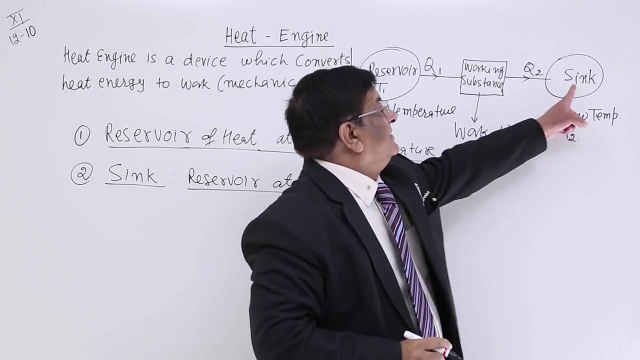 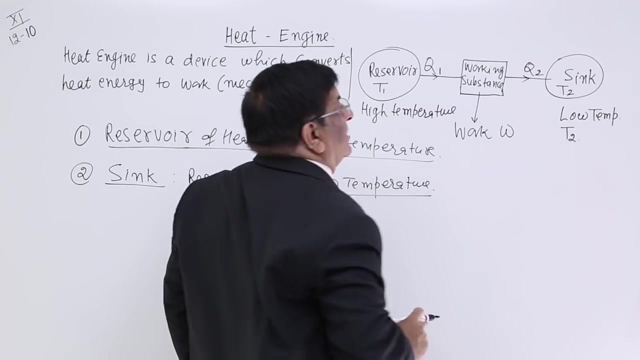 this is our reservoir now. the second thing is sink. sink is also a reservoir at low temperature. low temperature- here is scheme sink at low temperature- t2. now if we connect the two, the natural flow of energy is from high temperature to low temperature. sink again has got the same type. 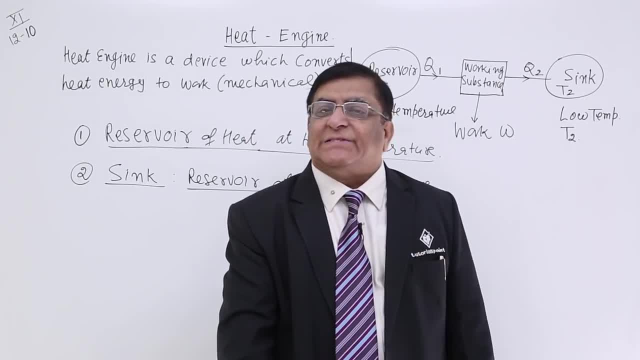 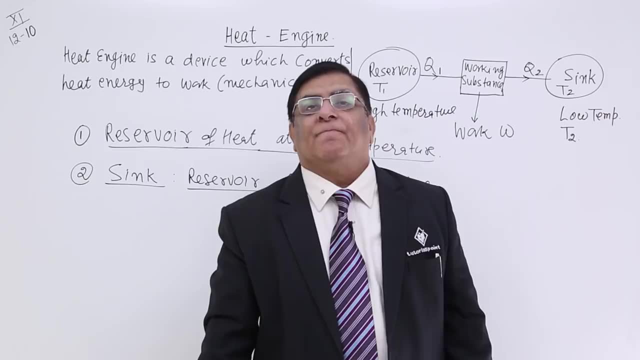 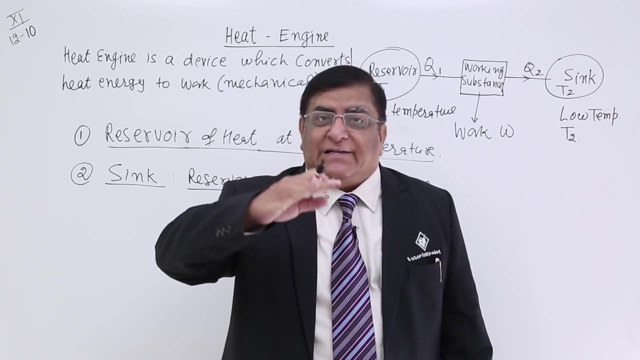 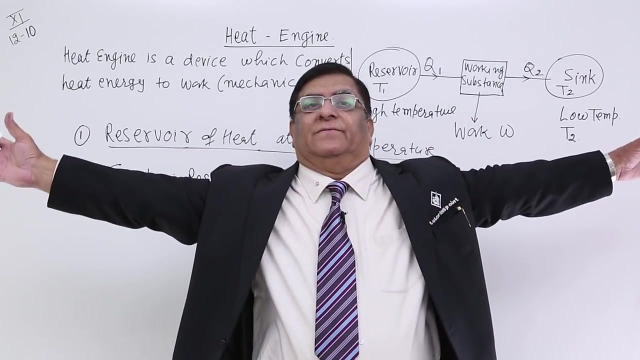 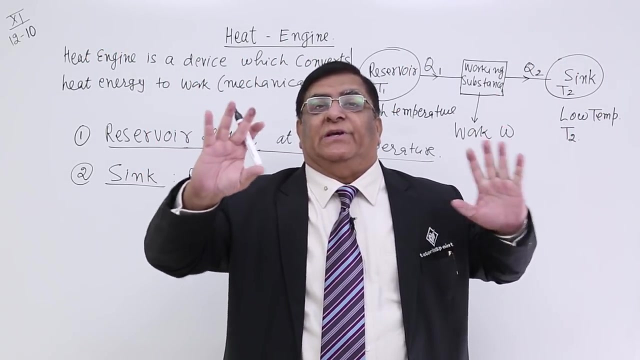 of characteristic. whatever heat you pour into it, its temperature will not rise. that is a ideal sink. let us see how it works. like if you keep on pouring water in the sea. does it level rise? no, that is a ideal sink. similarly, the atmosphere. if i, this atmosphere has certain temperature, say 22 degree at present. 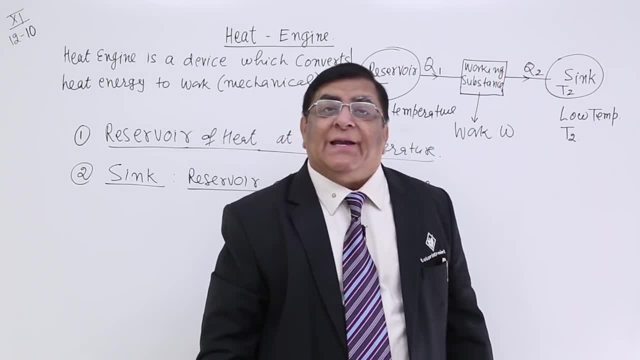 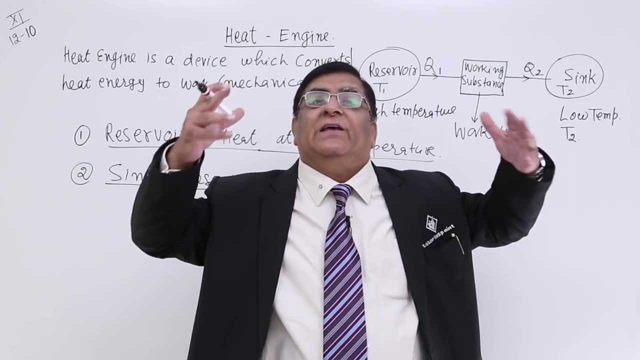 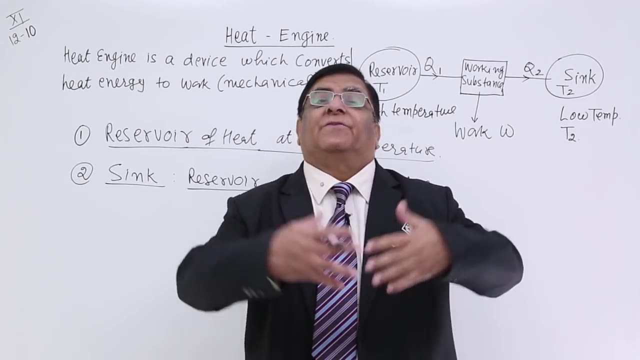 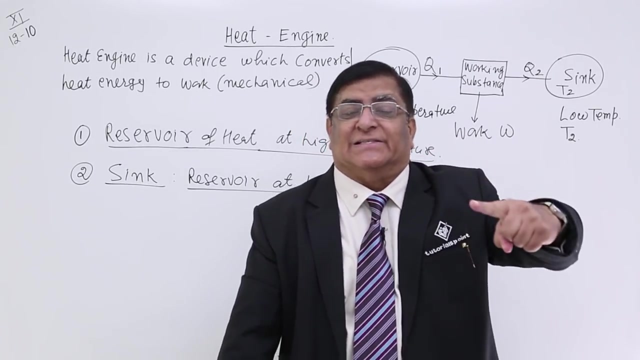 a motorcycle comes here and goes there again. i measure it after a minute or two. i find it is 22, because the total air contents are very, very large compared to the hot gases released by the motorcycle. so this is a very large reservoir. this is a sink. what is the job of a sink? we can reject heat in the sink. what is the job of? 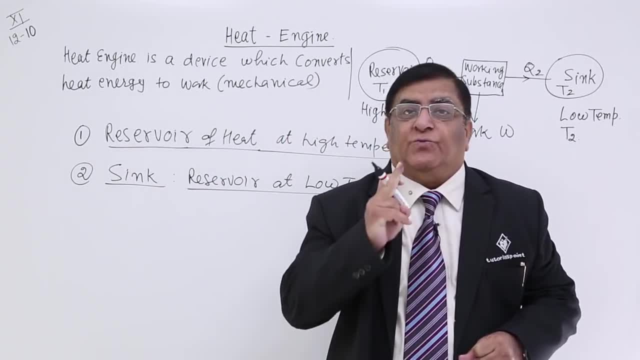 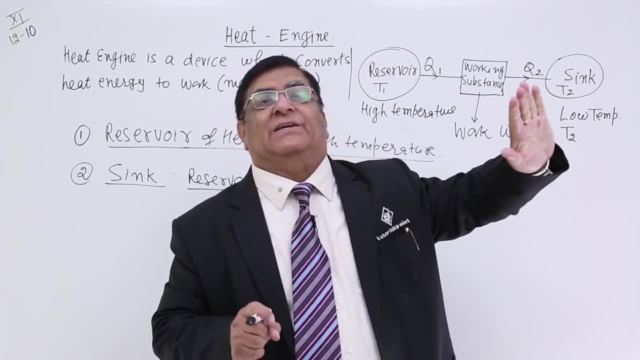 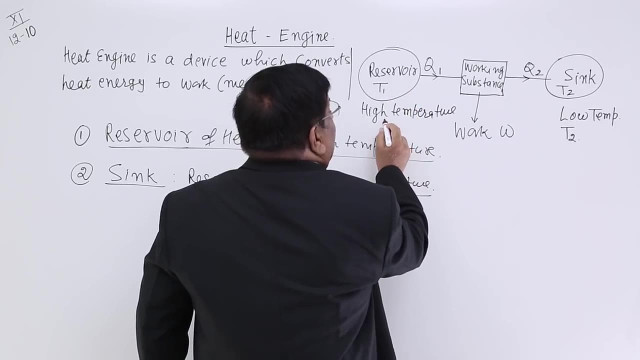 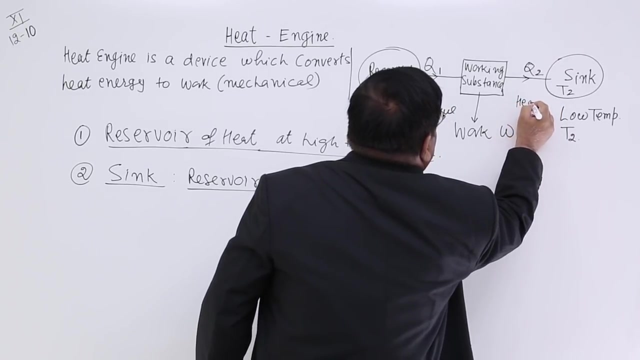 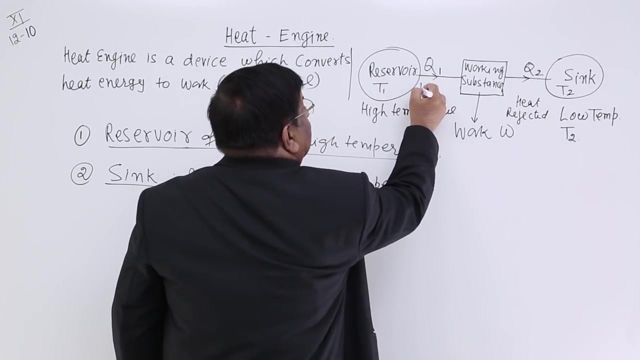 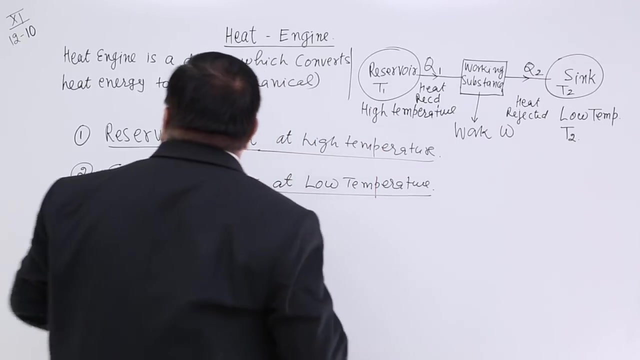 reservoir. we can take out heat from the reservoir. so we take energy from the reservoir and we can reject heat which is not used. that heat is rejected into reservoir. so this reservoir, energy taken from here, and this is energy rejected, heat rejected. okay, this is heat received. now, third thing is: 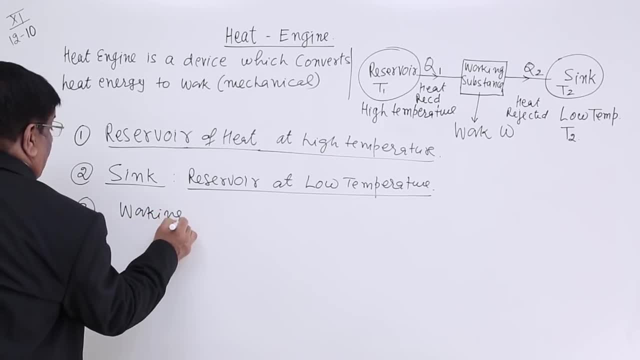 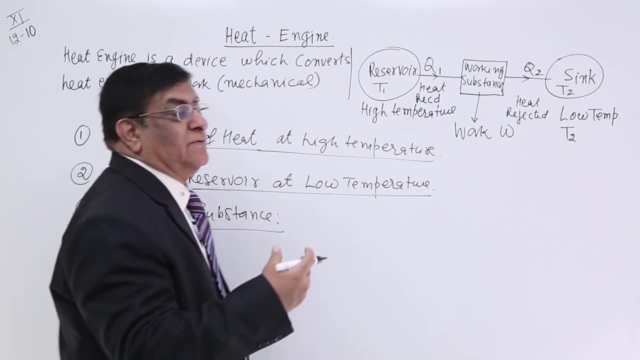 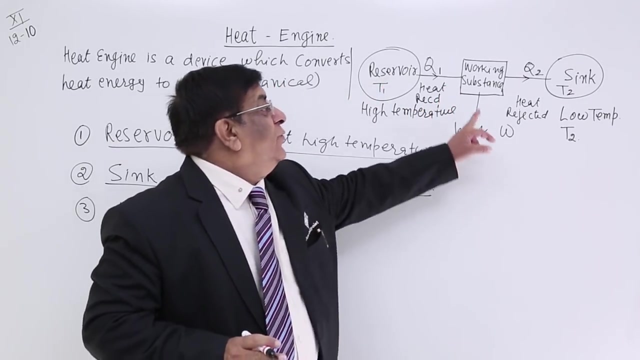 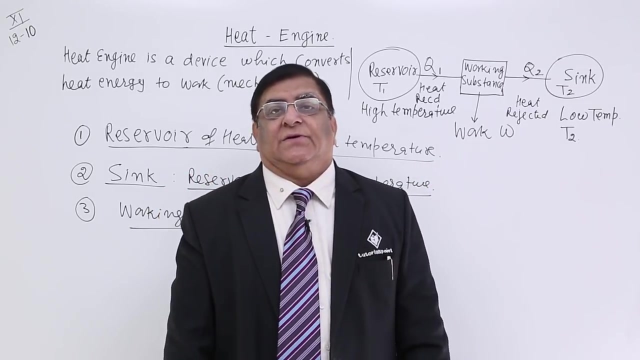 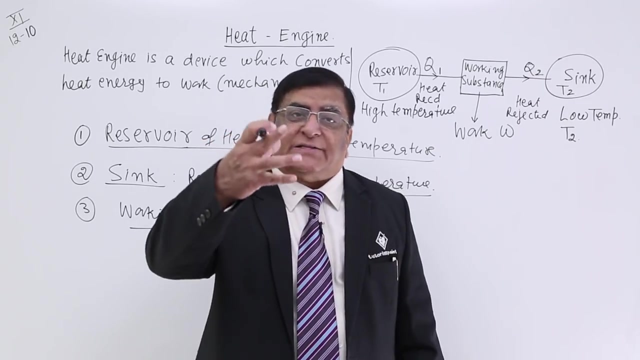 working substance. so what is the working substance? working substance is that substance which we are revising. we are using it for taking out heat from here, doing the mechanical work and rejecting heat to the sink. for that we choose a working substance like gases. the petroleum we burn, we get the gases co2, h2o, etc. 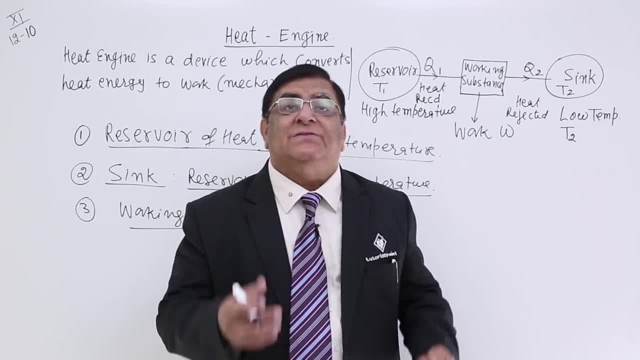 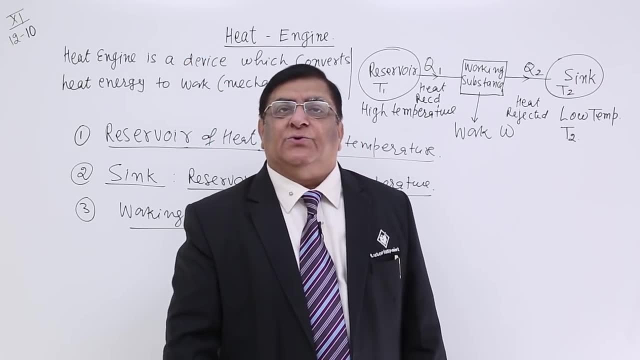 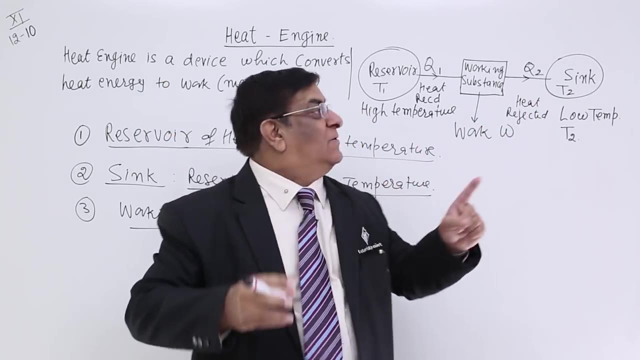 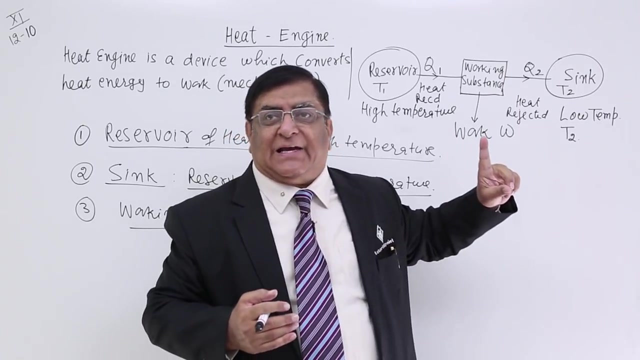 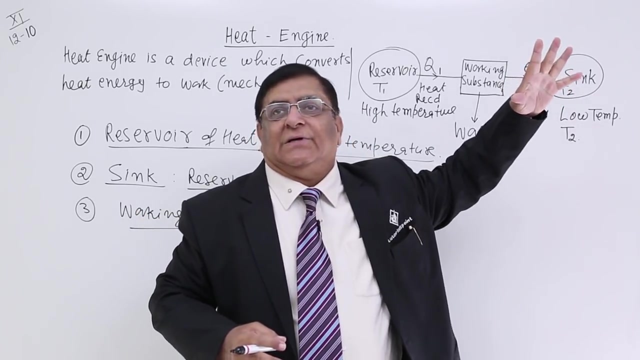 that mixture. that is our working substance in motorcycle and car. in other things, working substance may be different things. what does it do? it takes heat from the source. expand. when it expands. what does it do? do the work move the piston? that is expansion work is done and after that it is going out from the silencer that is rejected to sink. so that is our working. 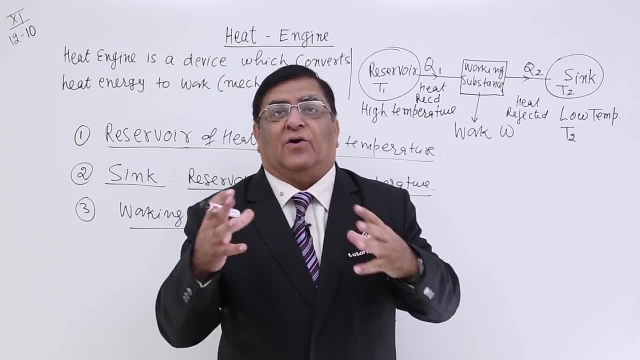 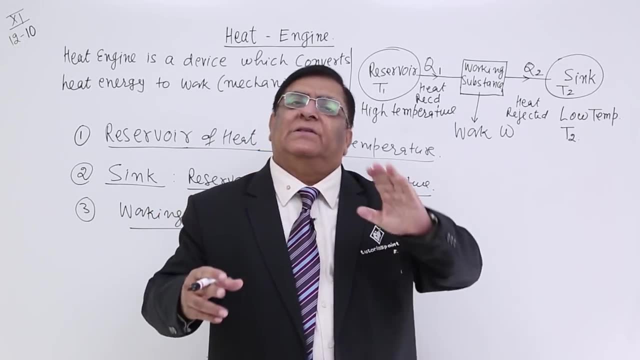 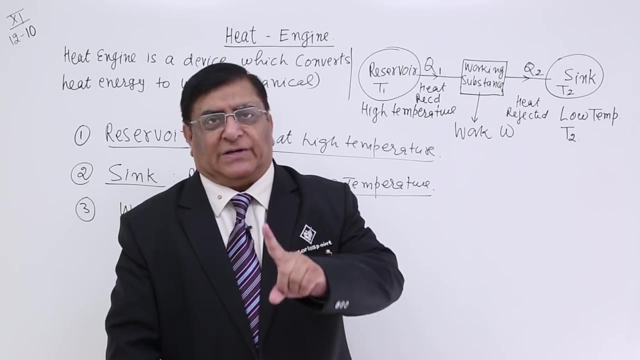 substance? what the hot gases, the burnt hot gases? in refrigerator, it is freon which is our working gases. in many other examples there will be different things, like in steam engine, it is steam which is our working substance. so that is our working substance. what does it do working? 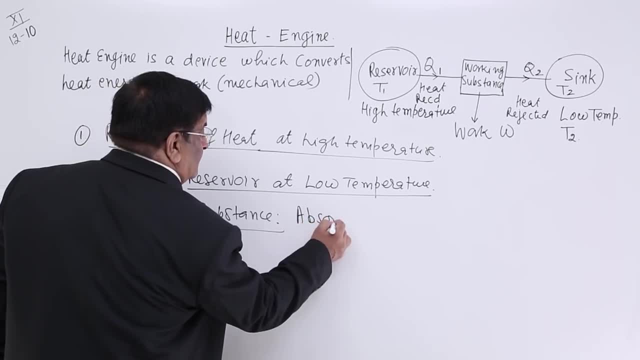 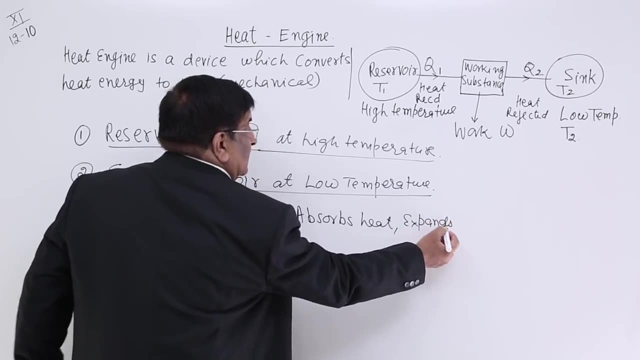 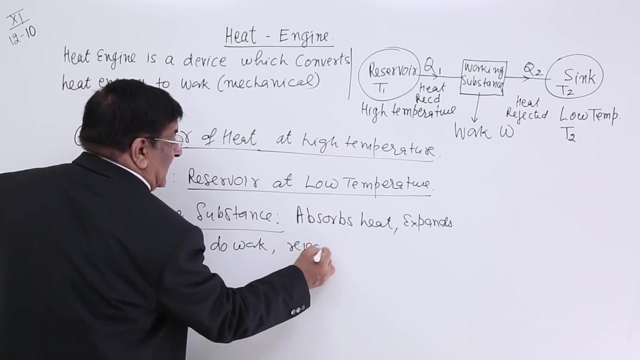 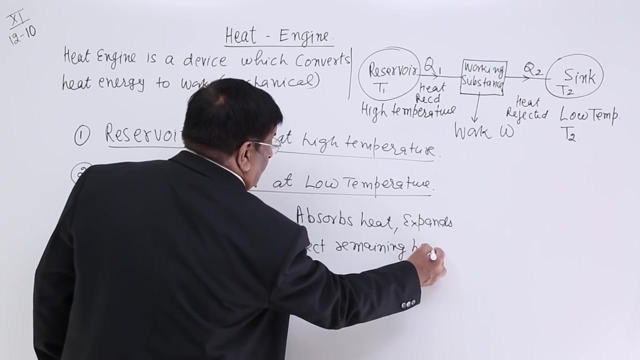 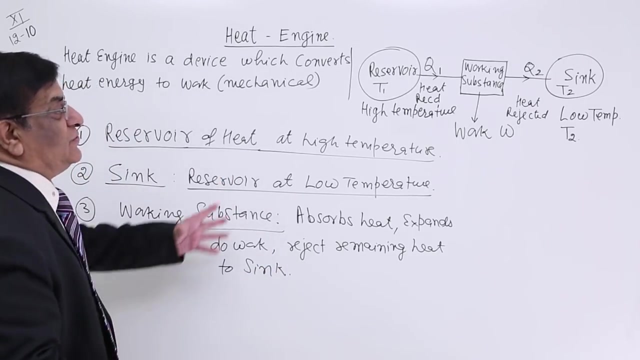 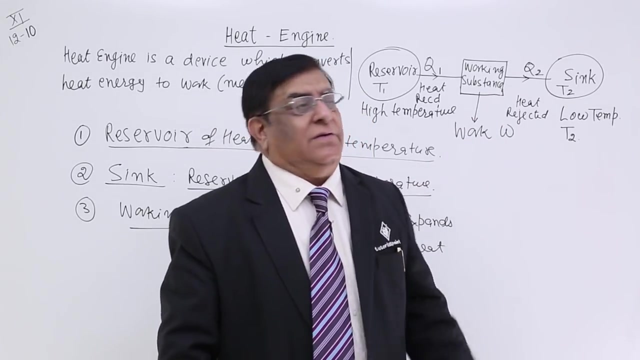 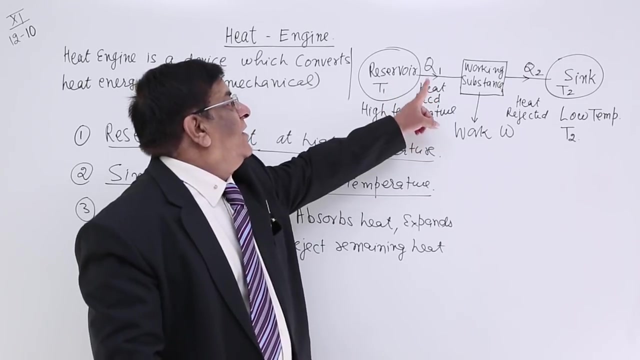 substance. it takes heat from the source, expand. when it expands, what does it do? it takes heat from our working substance, absorbs heat, expands, that is, do work and reject remaining heat to sink. this is working substance. doing so, these three things together makes an heat engine ok. here this working substance convert. it is taking heat from the reservoir q1. 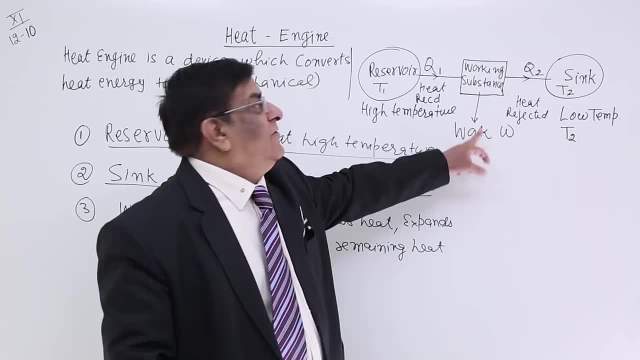 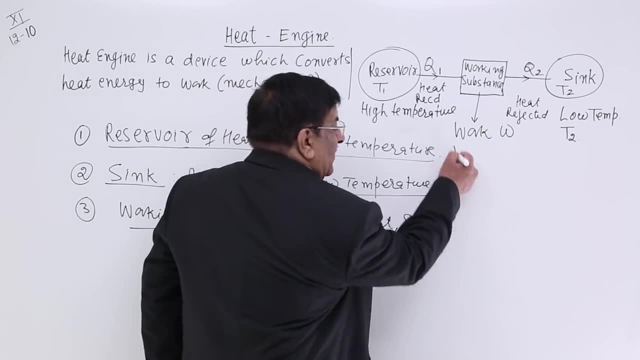 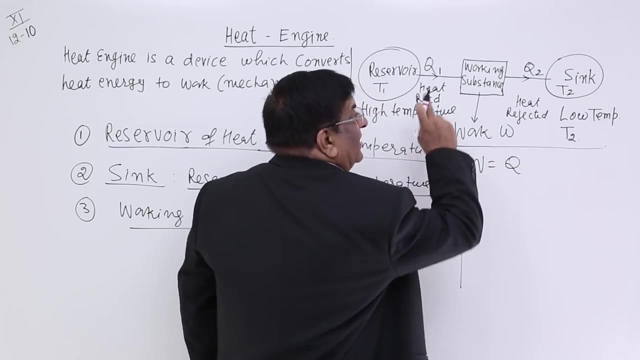 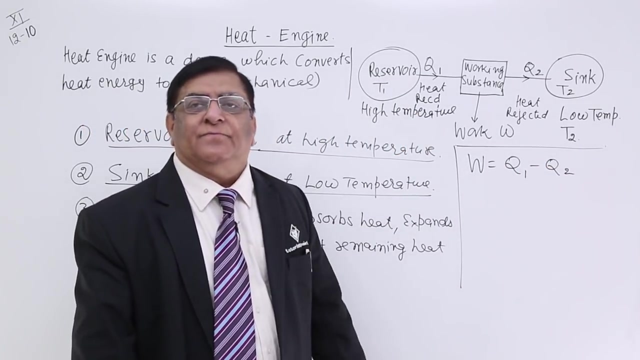 doing certain work: W, and rest of the heat it is rejecting to the sink. so how much work is done so I can write here: work done, work done? W is equal to change in energy: q1 minus q2. very simple, this is work done by the engine right now. how? 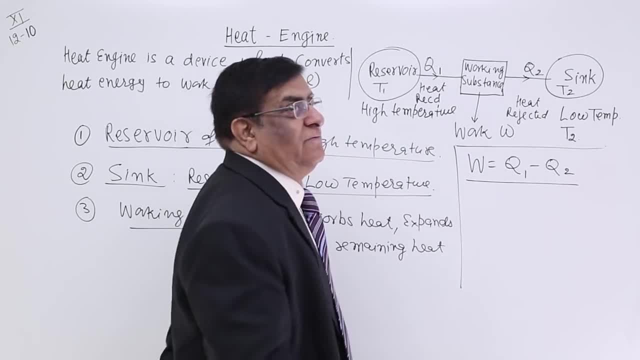 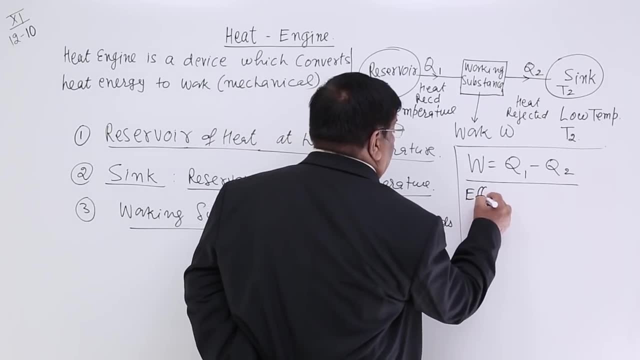 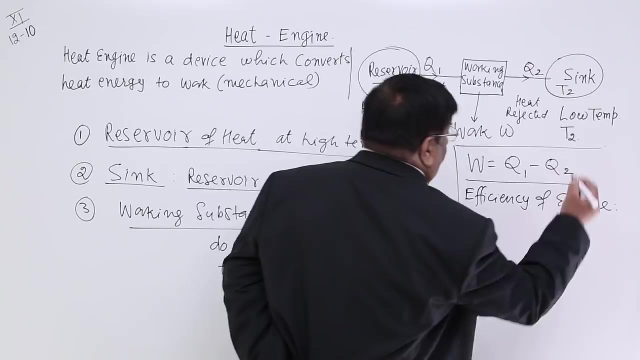 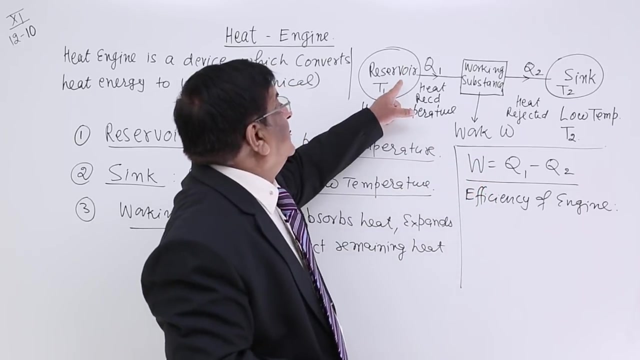 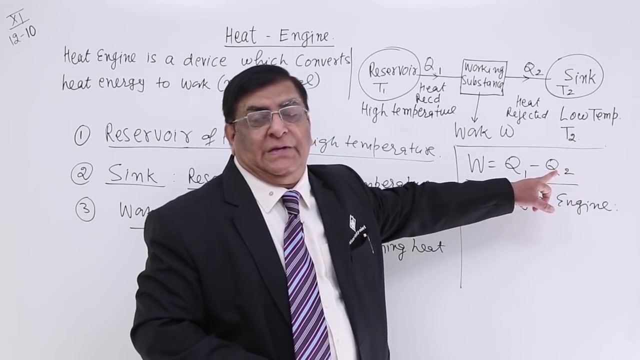 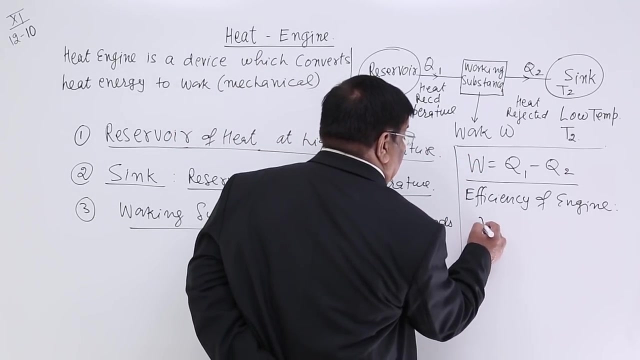 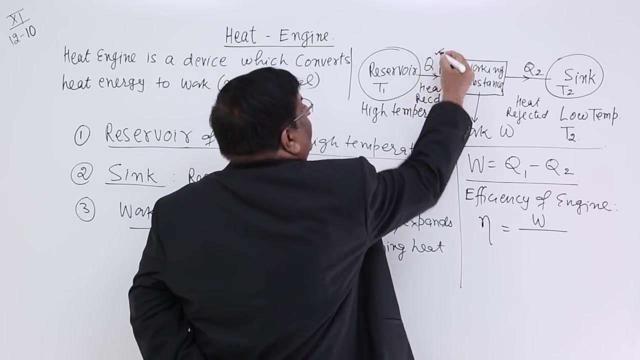 good is this engine that we measure in the terms of efficiency of the engine. I am getting the work done. W for that. they should give the heat q1. this should be high, this should be low and did this gives me efficiency. so efficiency is eta, is the work done and how much heat is taken from the reservoir q1. so if I take heat, 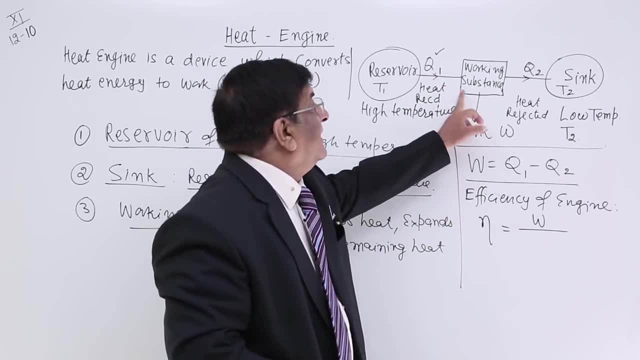 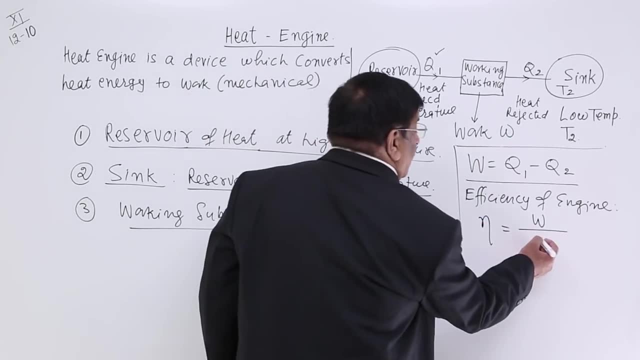 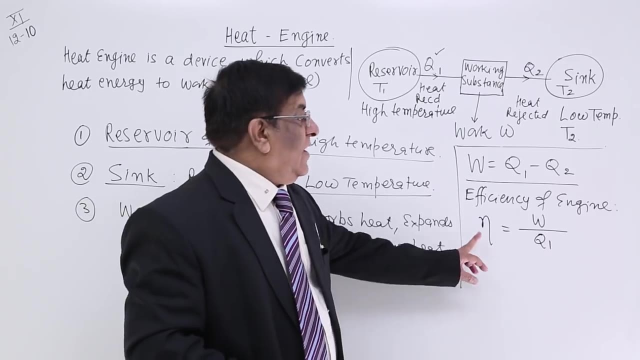 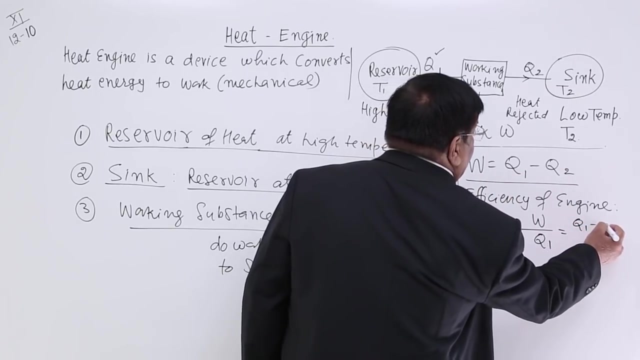 q1 from reservoir, then only I can convert a part of it into work done, W. so this is W upon q1. this is efficiency right now. here W is equal to W is equal to q1 minus q2, so I can write it q1 minus q2 upon q1, because for doing 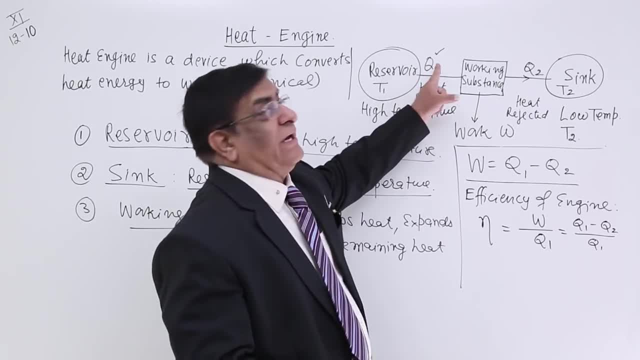 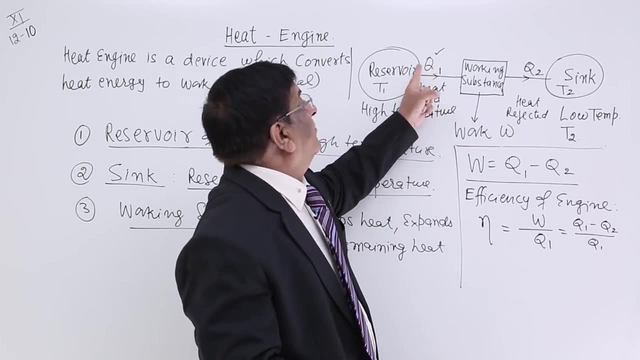 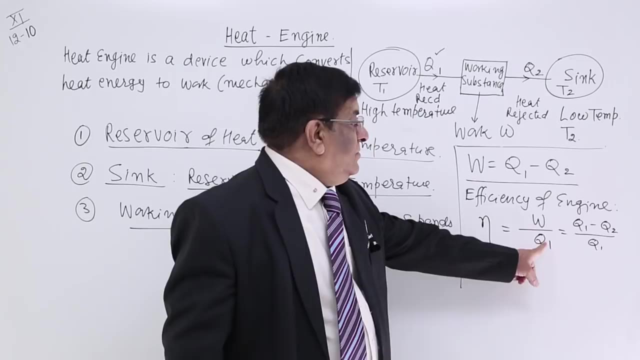 the work W. this is the quantity I have to take out if I want to to, if I want to work to W, then I will have to take out from here to q1, so that much energy we have to draw from the reservoir. So this energy, If I am drawing 100 joule from here and doing 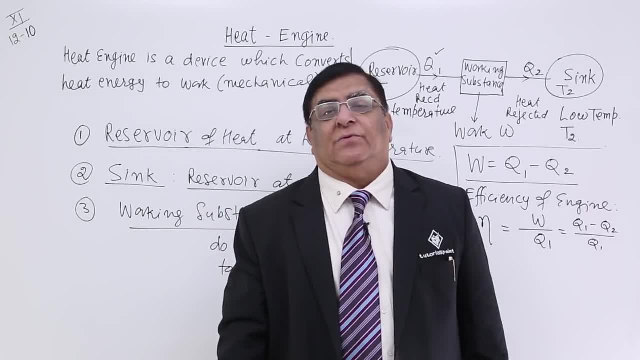 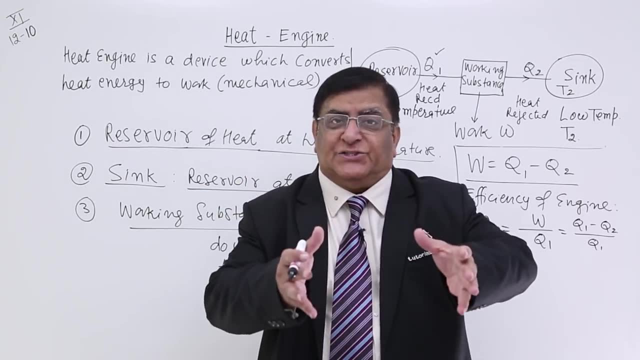 a work of only 20 joule. What is the efficiency of my engine? 20 upon 100.. If I have another engine, I take out 100 joule from here and the work done by this engine is 30 joule. 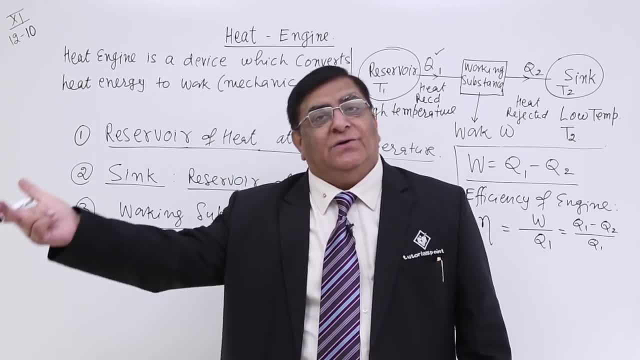 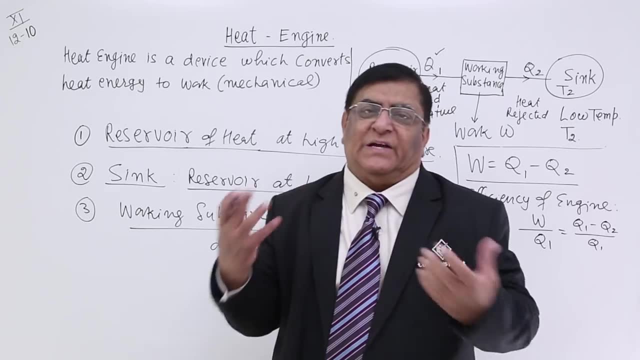 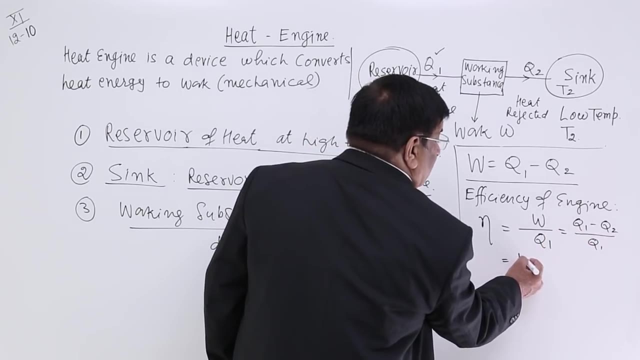 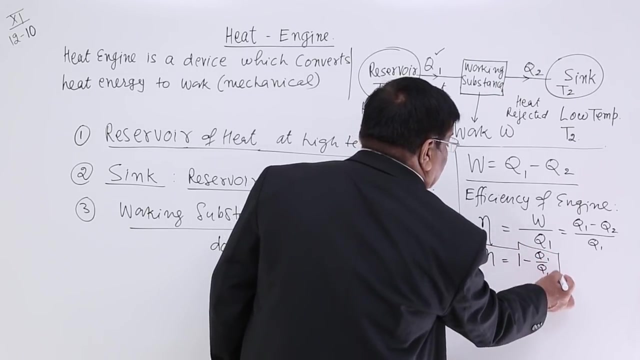 Then I will say its efficiency is 30 upon 100.. So the relation of work done to the heat taken, That is efficiency here, And this is the formula, And this we can write as 1 minus Q2 upon Q1.. This is remember, please. this is efficiency formula. 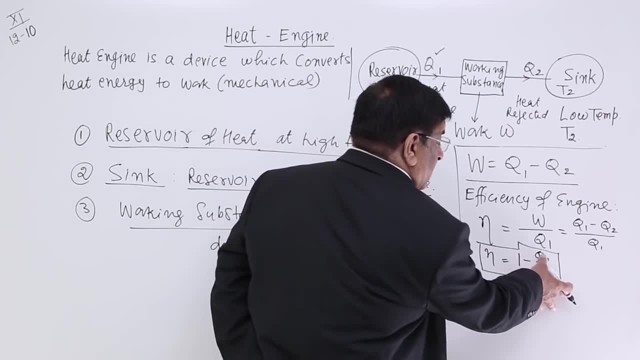 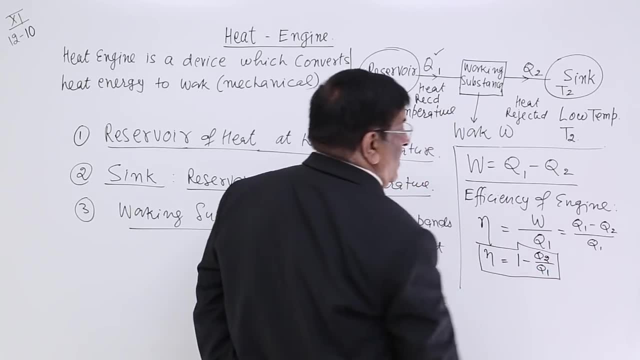 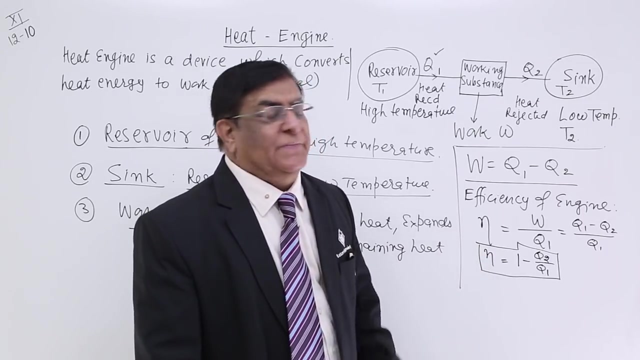 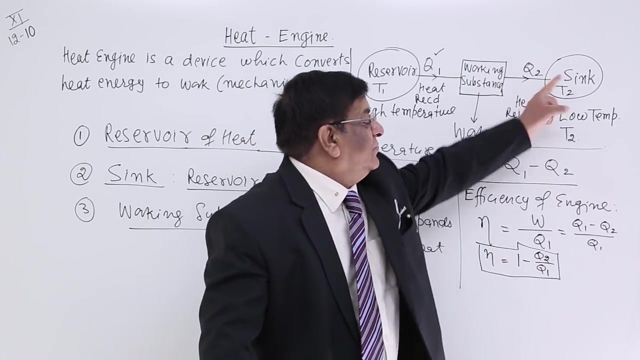 Now this is 1 minus Q2 upon Q1.. 1 minus Q2 upon Q1.. This is efficiency relation. Now here, Q is what Heat given, Q1, Q2 is heat given to sink, Q1 is heat given by the reservoir. Now, 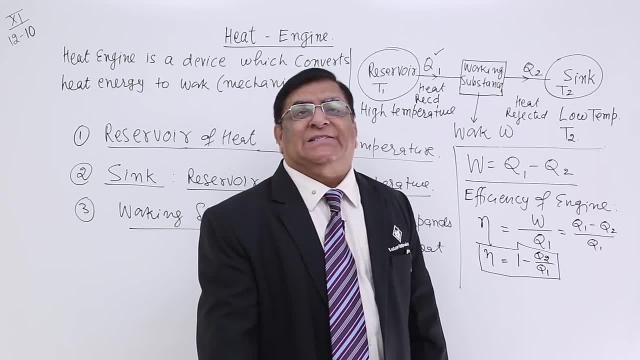 heat. we have a formula which says M S, Q1,, Q2,, Q3,, Q4,, Q5,, Q6,, Q7,, Q8,, Q9,, Q10,, Q11,, Q12,, Q11,, Q12,, Q11,, Q13,, Q14,, Q13,, Q14,, W S, T. T is what Temperature M is, mass S is. 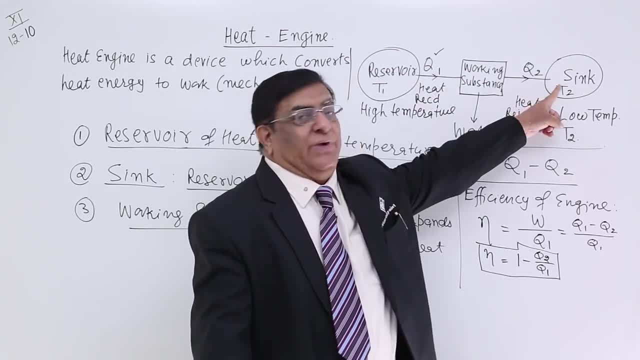 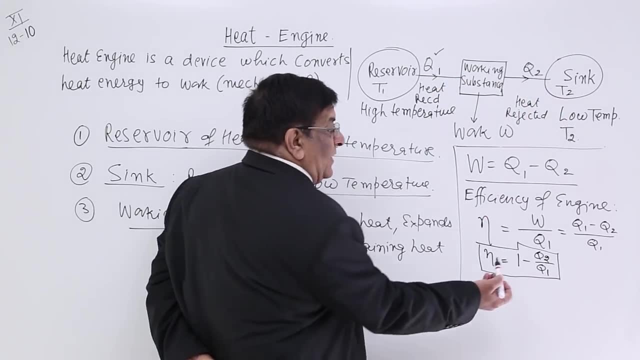 specific heat. The same gas is going here, So mass and specific heat is same. The temperature changes T1 to T2.. So here we can write as M S T2.. This we can write as M S T1.. And we: 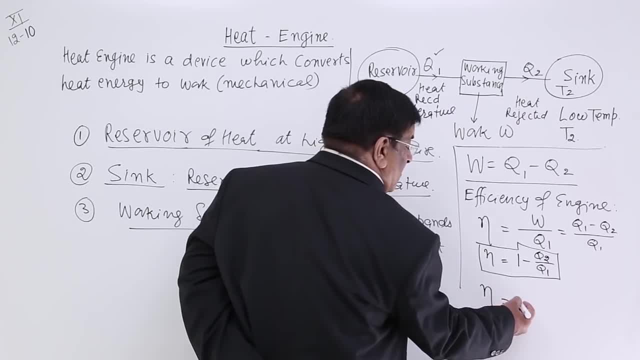 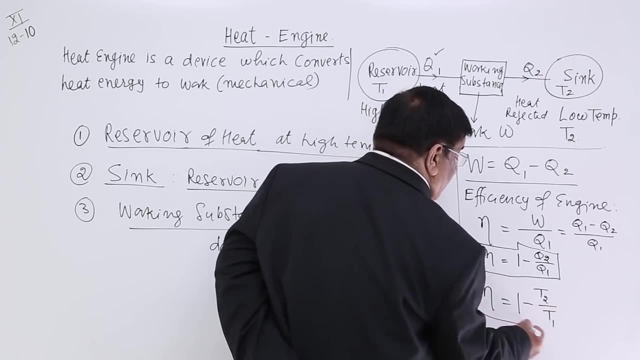 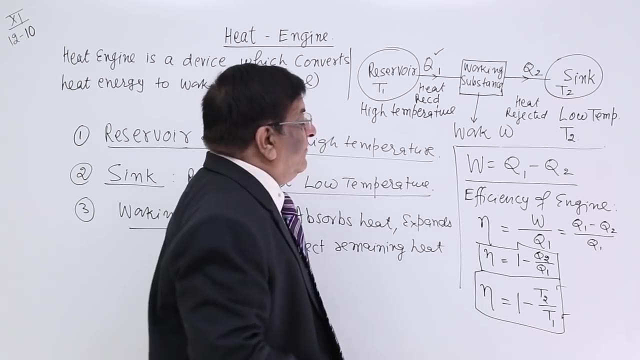 get the new relation of eta with. based on temperature, This is 1 minus T2 upon T1. Because Because with our thermometer we can measure temperatures, So this is more practical formula. we cannot measure the heat taken out or the heat going. 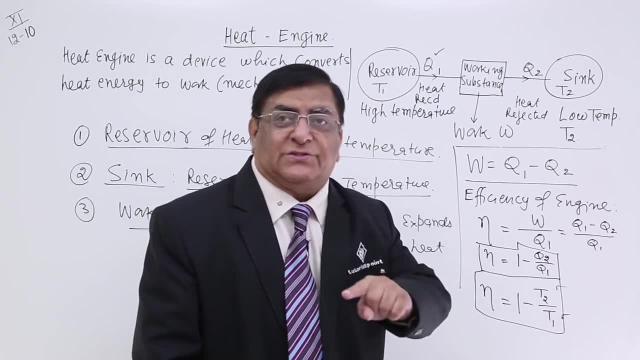 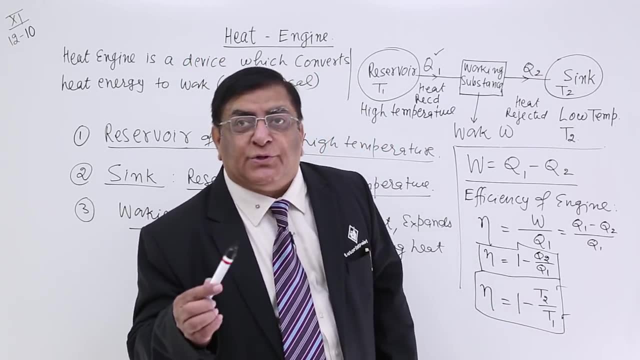 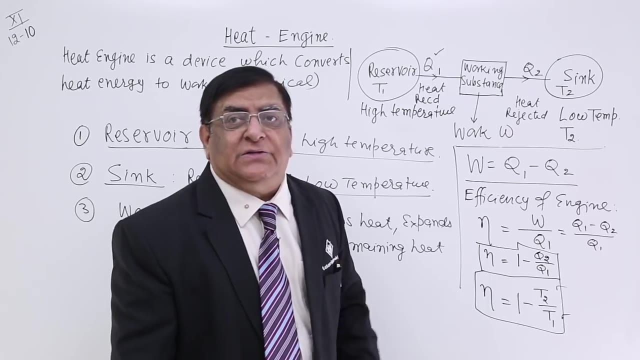 to the sink Temperature we can measure. If a motorcycle is going here, I put the thermometer here in the air, that gives me T2.. If I put it thermometer with the engine, that gives me T1 and that shows me efficiency. If I convert the full heat, full heat, into the work, then Q2 will be 0. and what will be? 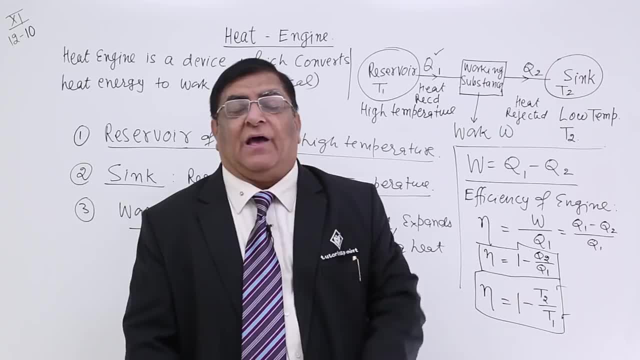 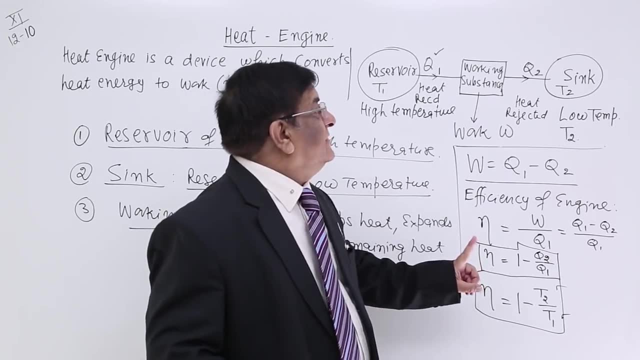 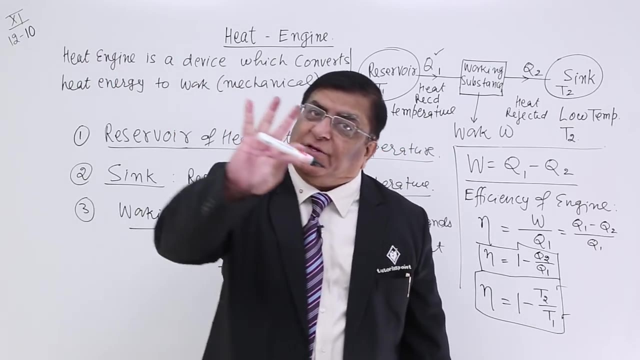 efficiency 1. That is the maximum efficiency which we never get. Why do not we get that full efficiency? Because we have to pass certain heat to the sink. If we do not, that means we are stopping the flow of heat. If we stop the flow of heat, work will not be done. 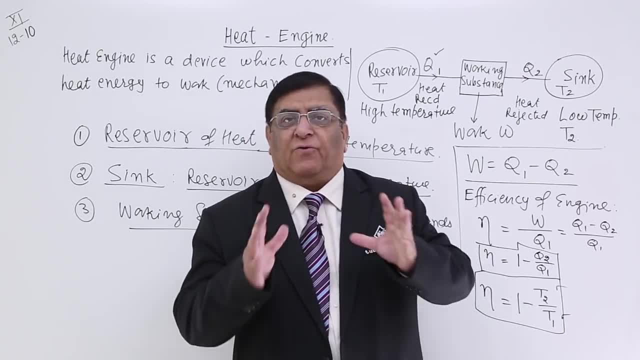 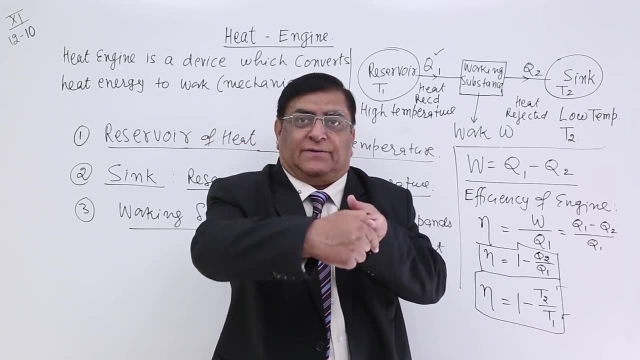 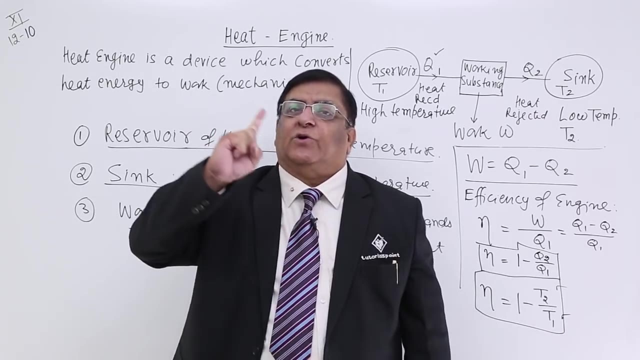 You see, once again, if I want to do a work with flowing water, like I want to run a turbine with flowing water, I want to wash my hands with flowing water. What is the first requirement? The first requirement is that water should flow. 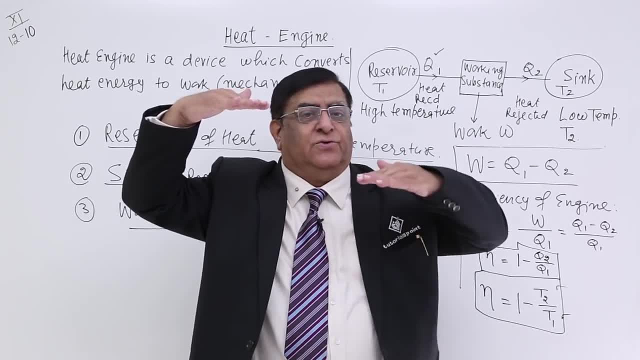 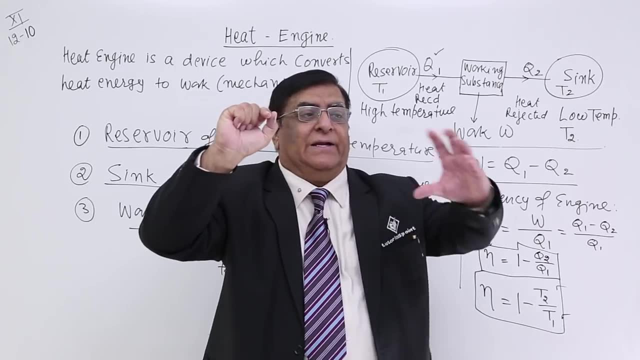 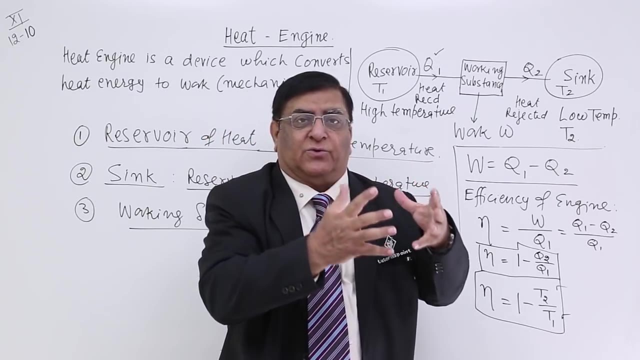 How the water flows from higher level to lower level. Now I have this higher level of water that is stored in the overhead tank. This is the bottom. I say I do not connect them because the water going in the sink, water going in the drain. 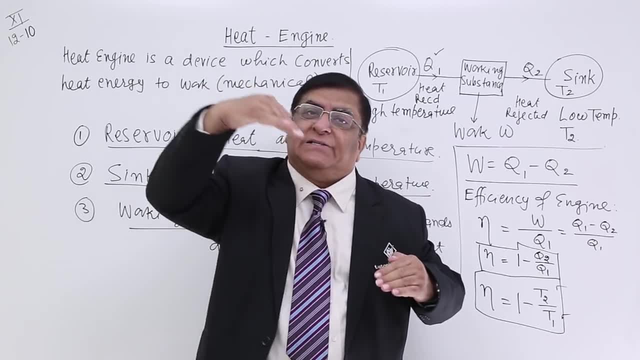 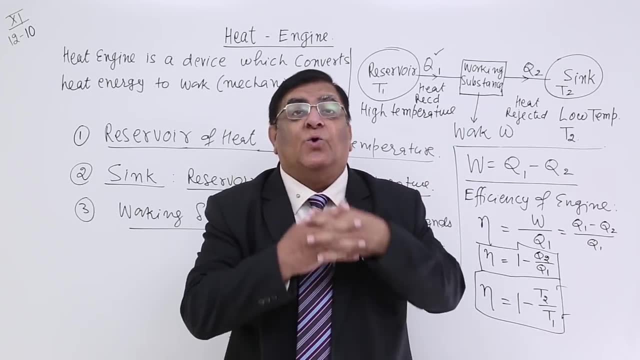 is of no use to me. So I stop this pipe and I stop the flow. If I stop the flow, the turbine will stop And I cannot wash my hands. also, No work can be done unless water is flowing. And what is the condition for water flowing? 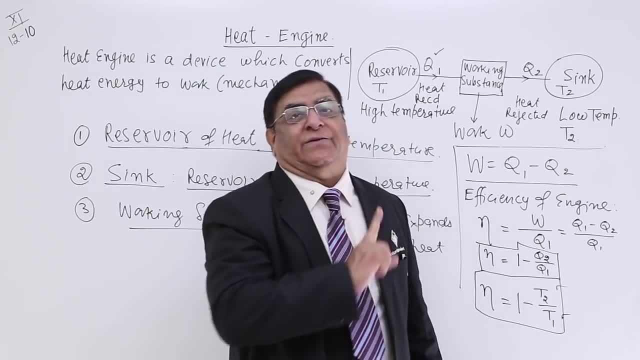 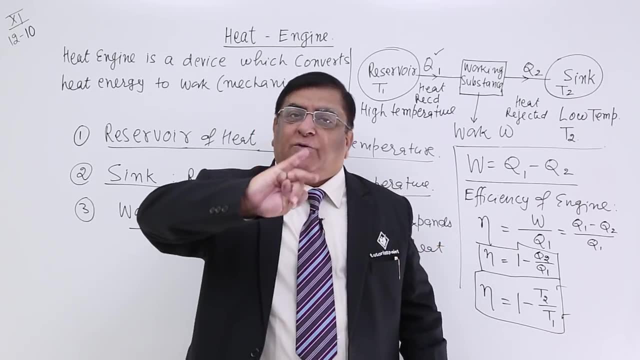 The drain should be open and some water must be going to the drain. If no water is going to drain, then what is the condition? The drain should be open and some water must be going to the drain. Okay, the drain water is not flowing. and if water is not flowing, then turbine is not moving. 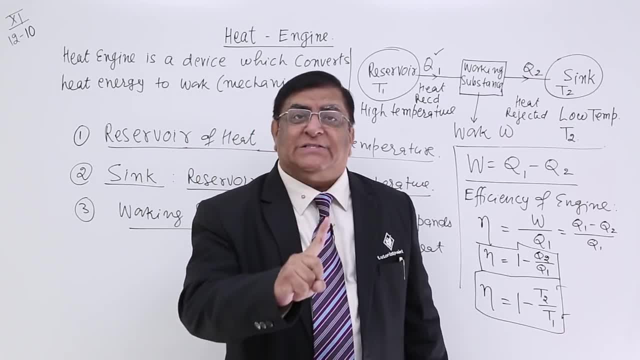 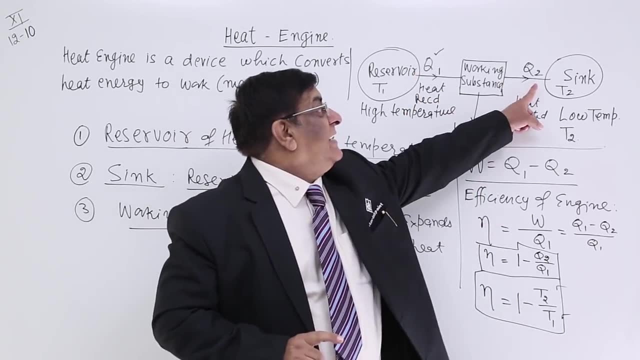 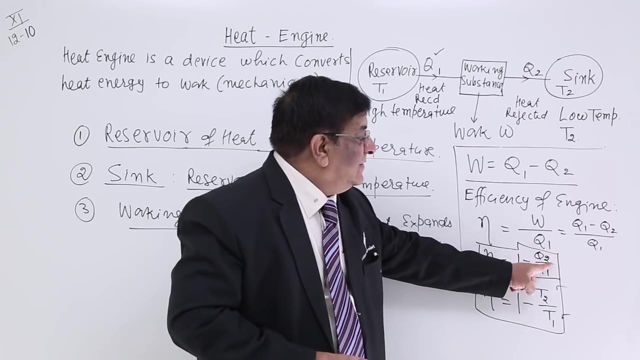 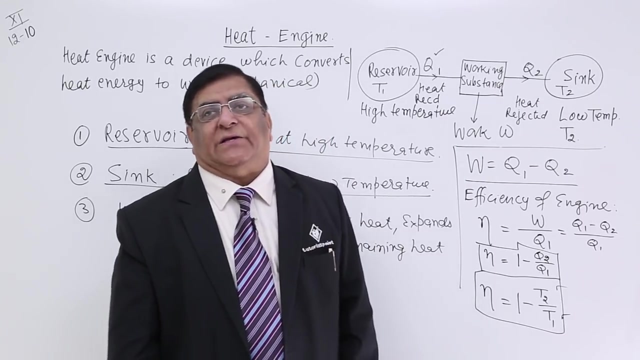 we cannot do any work. so it is compulsory that some water has to go to drain. that means some heat has to be rejected to sink. now, if this heat has to be rejected to sink, efficiency can never be one, and this is the principle of physics, thermodynamics. 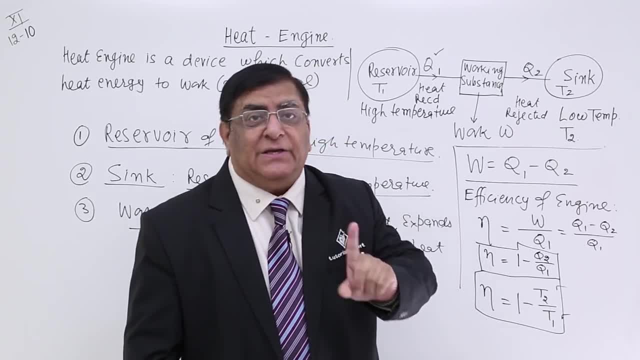 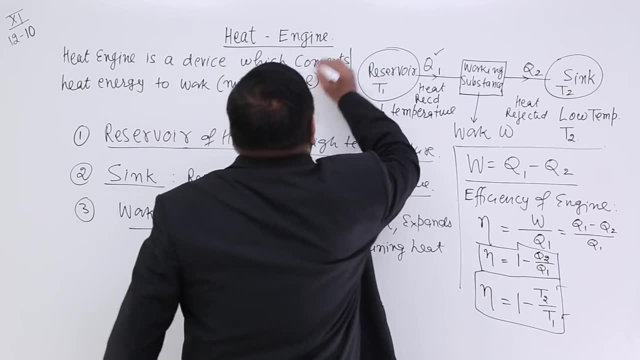 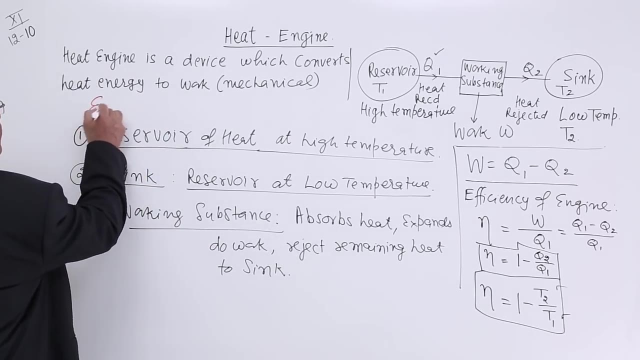 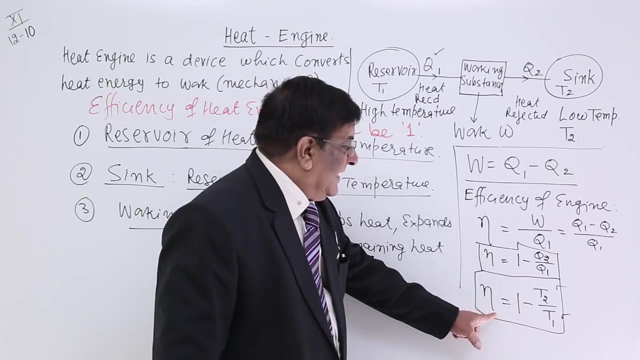 that efficiency of any machine can never be one. it will always be less than one, and this is in bold letters. efficiency of an engine can never be one. you you will also see here that if efficiency has to be one, this t2 must be zero. that means absolute. 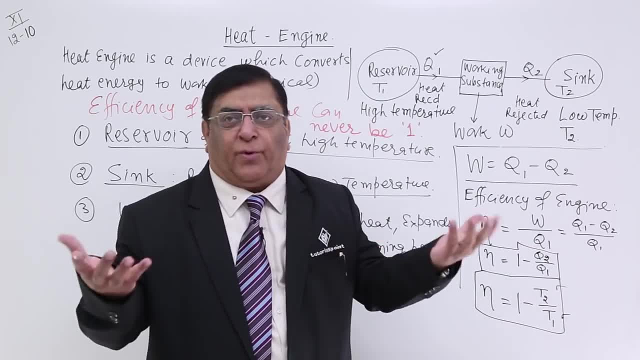 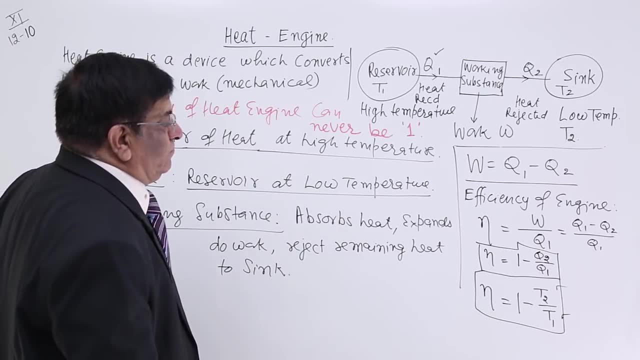 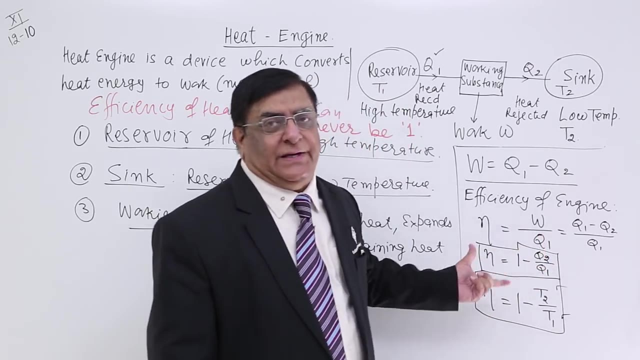 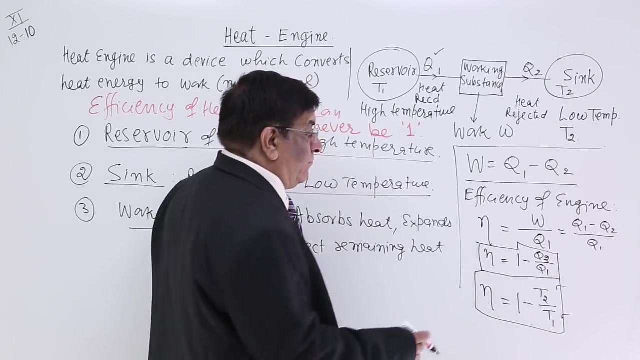 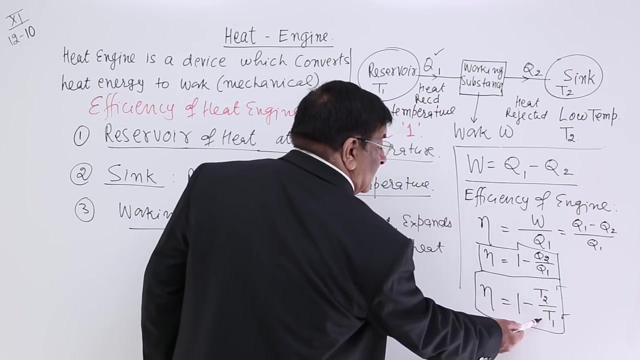 zero, that means minus 273, which is not possible. therefore, efficiency can never be one. so with this we get another very important feature, that is, which heat engine has more efficiency? the answer is: if t1 is large, then this will be a small quantity. minus small quantity will make it. 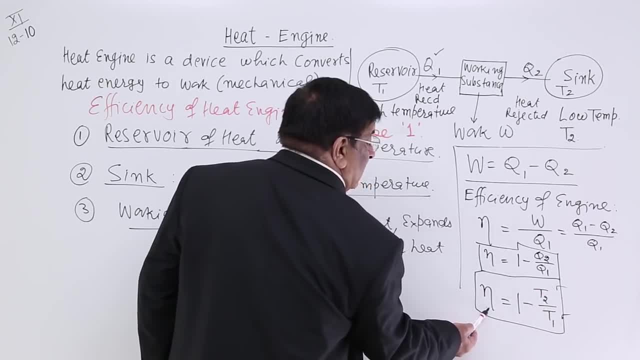 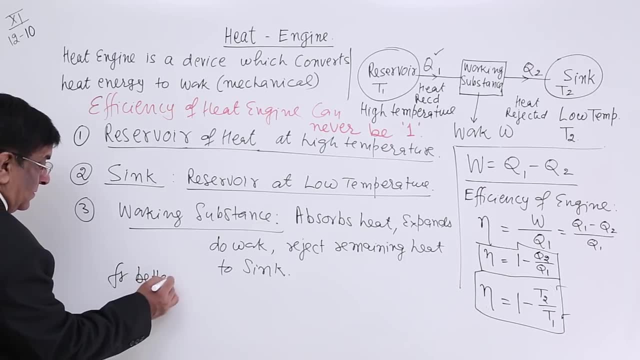 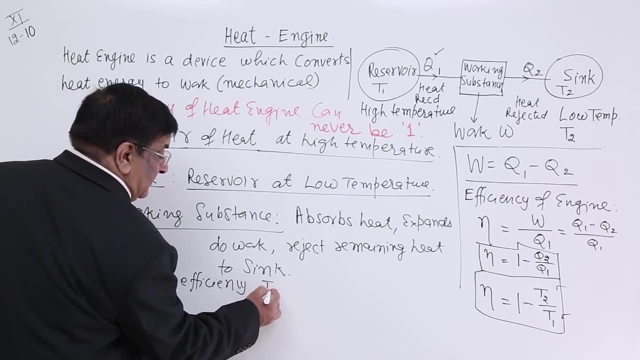 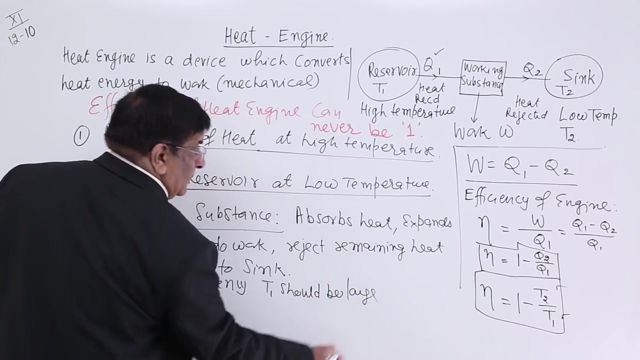 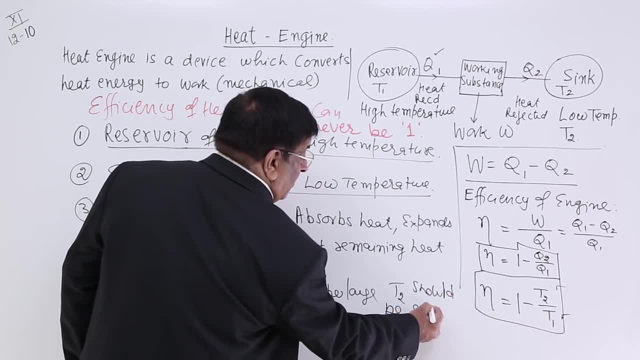 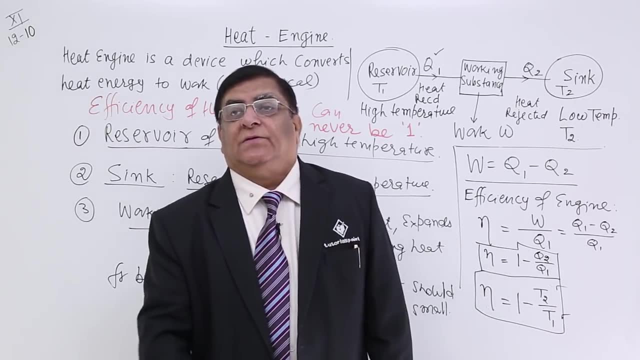 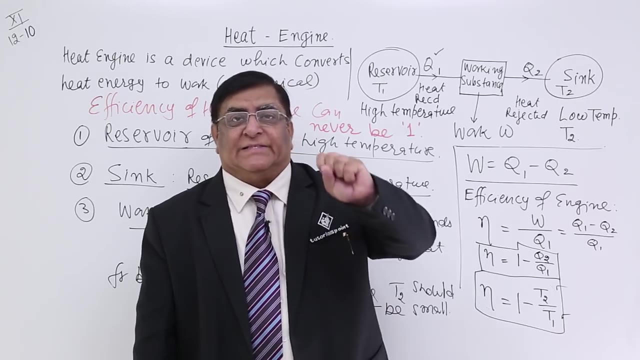 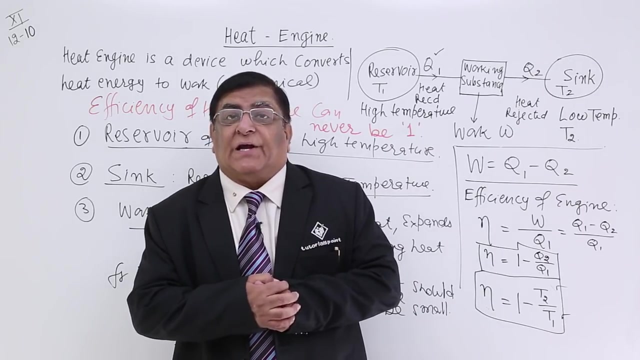 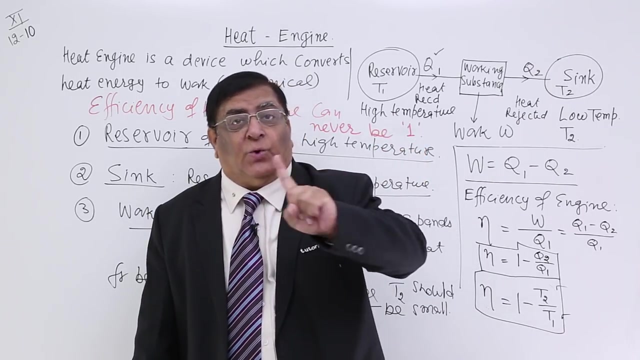 t2 should be small, as small as possible. t1 should be as large as possible. that means made that should be as hot as possible. you always try to find out whether engine is not very hot, because the hot engine, the efficiency decrease. no, in a design process, whenever design, 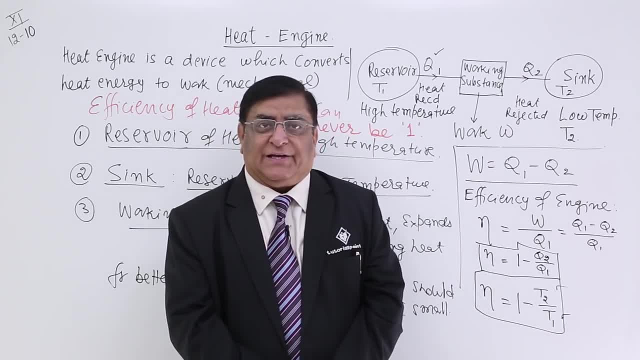 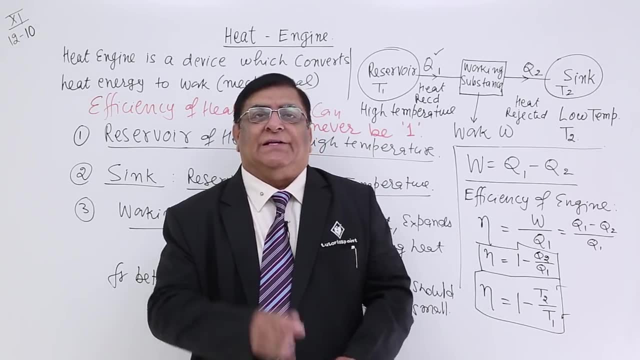 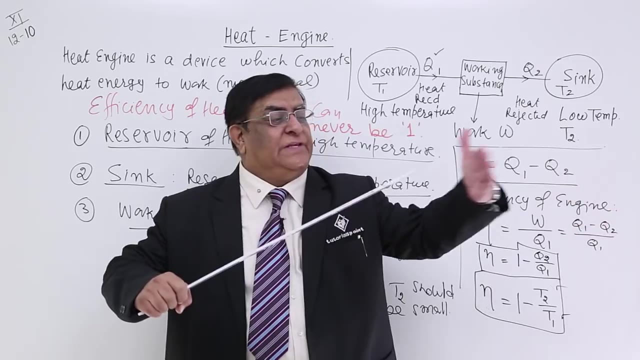 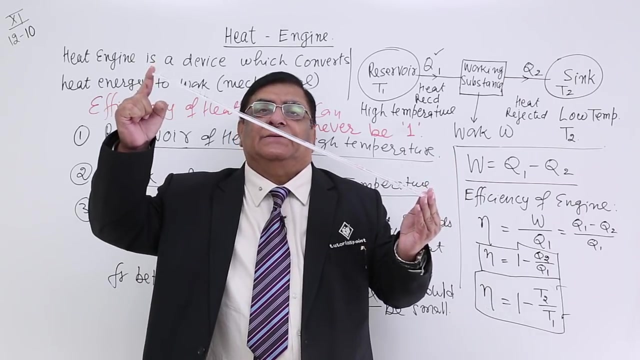 says my engine is working at 100 degree, other design says my engine is working at 200 degree, then always a design with 200 degree is more efficient, and that is very clear. if this is our atmospheric temperature, this is our engine temperature, this is 100 degree, energy will. 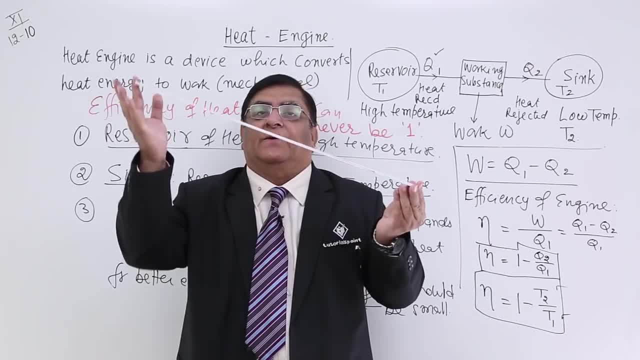 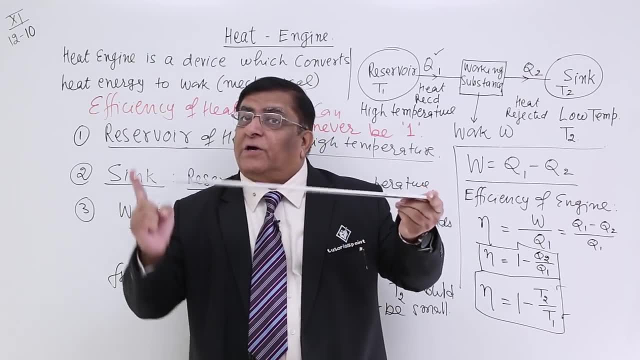 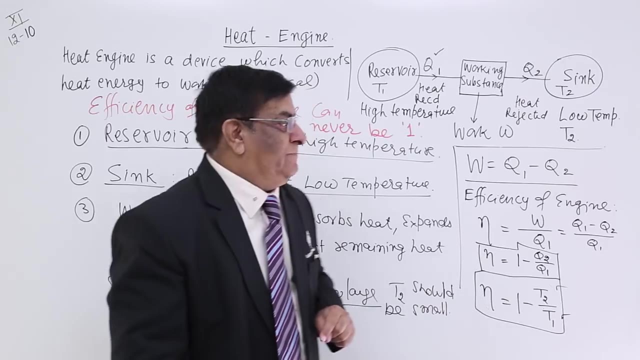 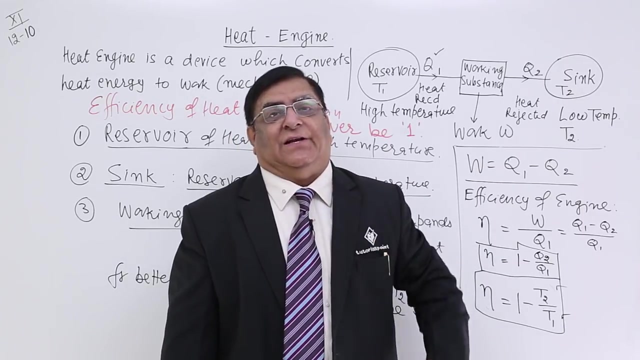 flow with this rate. if it is 200 now, energy will flow with this rate and this flow is faster, so hotter is the temperature of engine makes the engine more efficient. that is one thing. with this reason you can differentiate between petrol engine and diesel engine. the petrol engine works at: 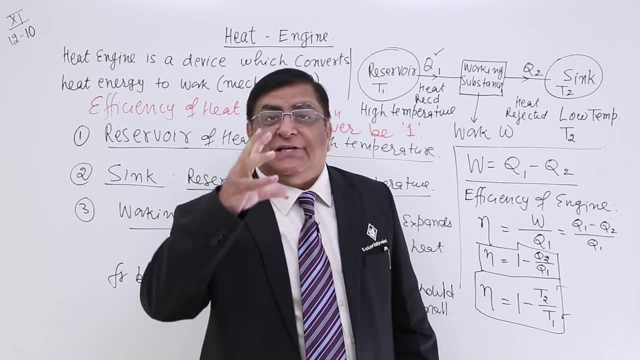 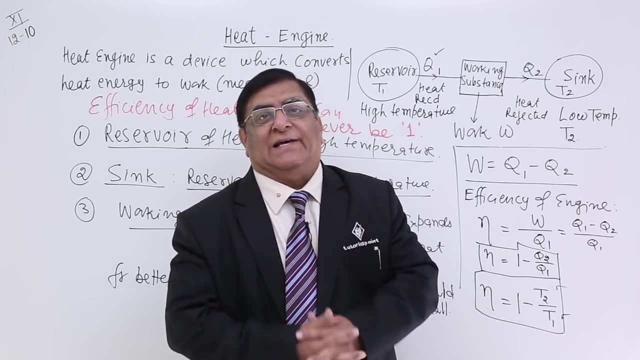 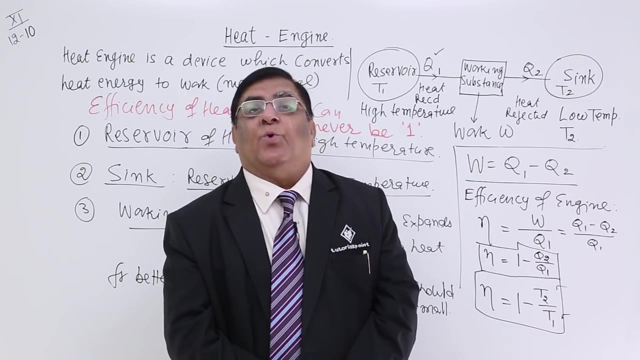 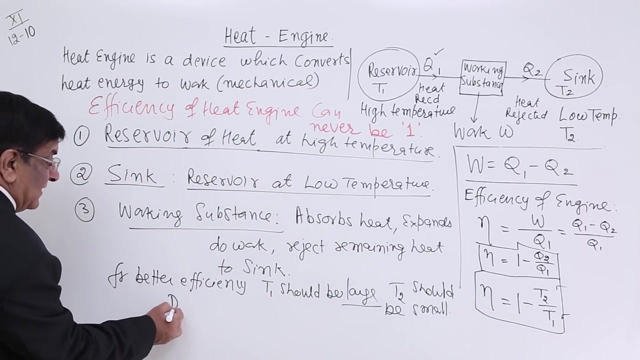 400 degree, while the diesel engine diesel burns at more than 700 degree. so the temperature inside where the gas is burning for diesel is higher. the t1 for diesel engine is higher. so which is the more efficient engine? answer: diesel is the more efficient engine. please remember why diesel is more efficient. 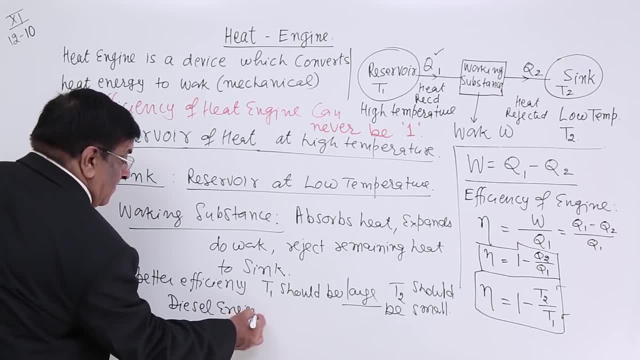 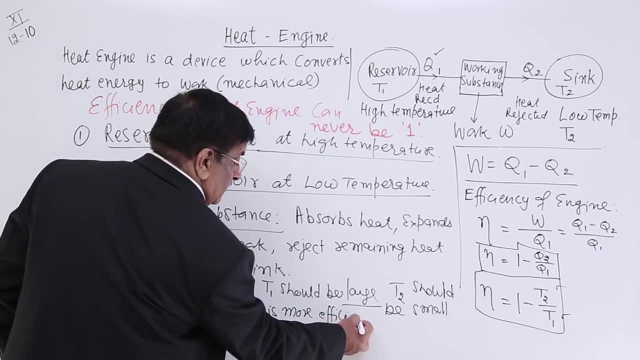 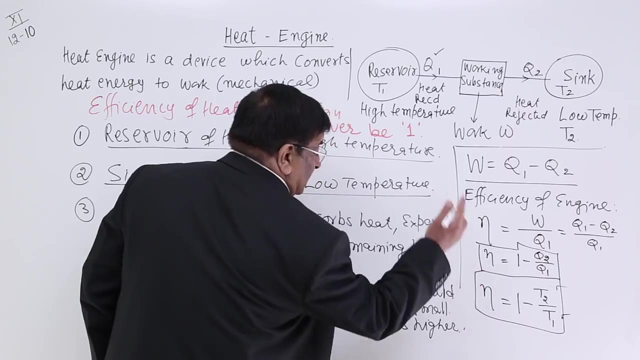 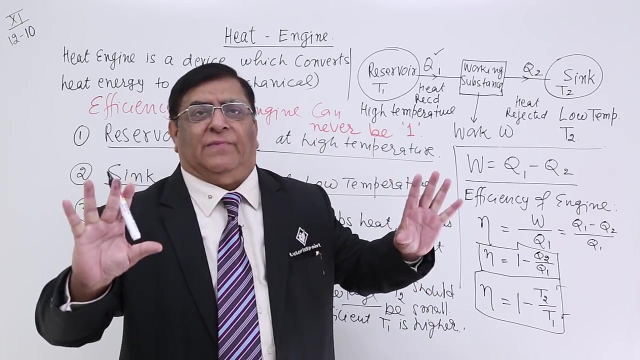 engine. diesel engine is more efficient, why t1 is higher. please remember this reason. but this is not the only reason why the fuel engine burns at more than 600 degree. This is only for efficiency purpose. we are not talking about the environment damages done by diesel or done by petrol. that is a separate issue. 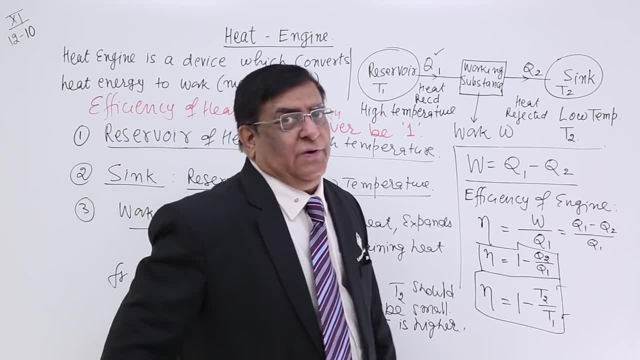 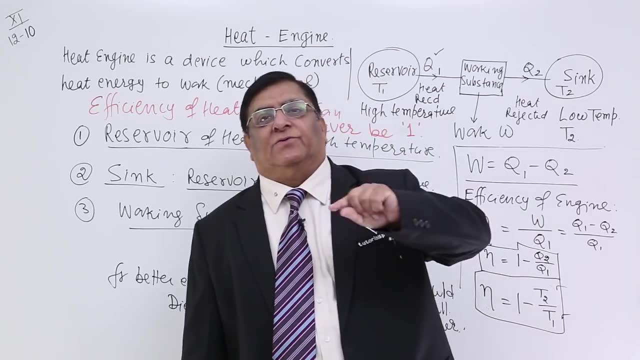 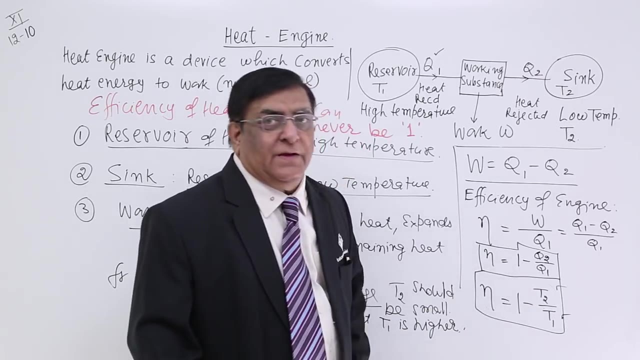 As far as efficiency is concerned. so you will find that with 1 litre diesel, the car can run a larger distance compared to 1 litre of petrol. this is the reason for that. Now the second reason: T2, T2 is what? 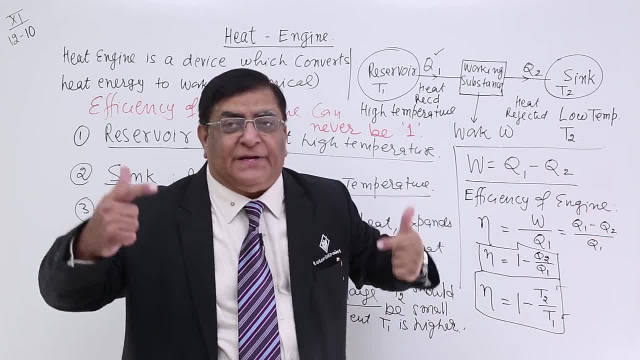 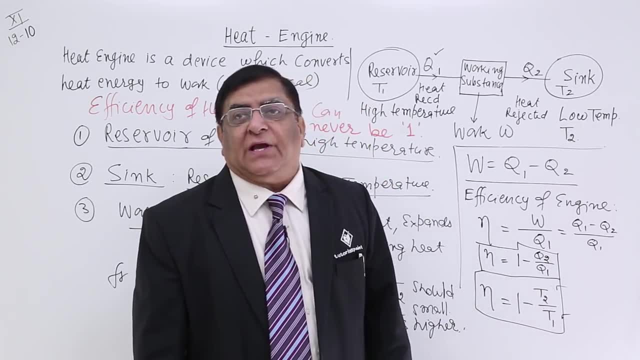 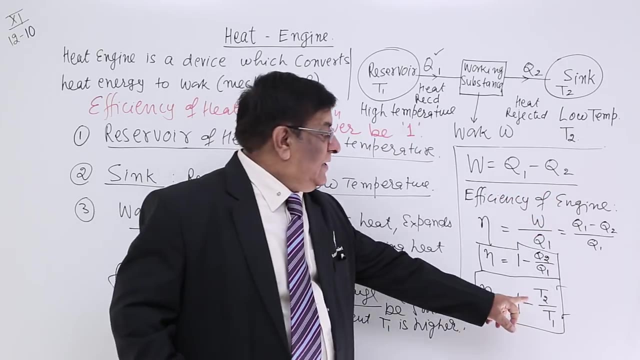 Temperature of the sink, temperature of the atmosphere, temperature of the surrounding. If it is low, efficiency will be high. How it can be low? Answer: in the colder countries. So in the colder countries the atmosphere is colder, T2 is colder. 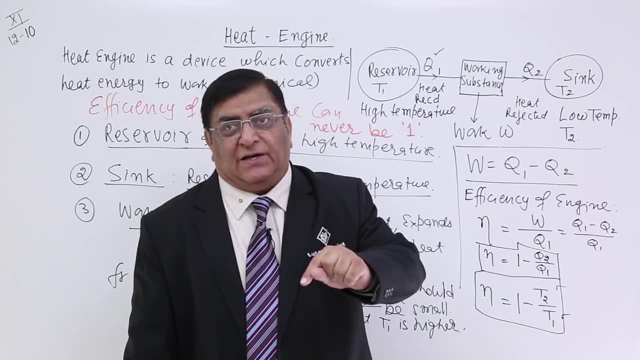 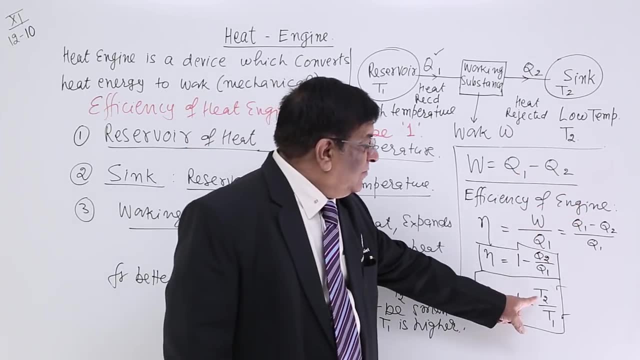 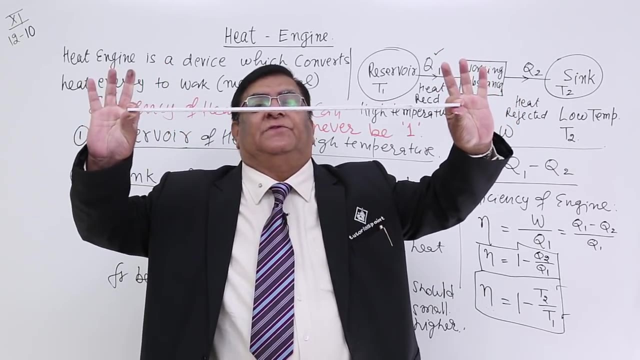 So the same engine which work in India has less efficiency. See if it works in England. it has more efficiency because the atmosphere temperature is less Here. this is T1,, this is T2, if they are equal there is no flow of energy. engine will not. 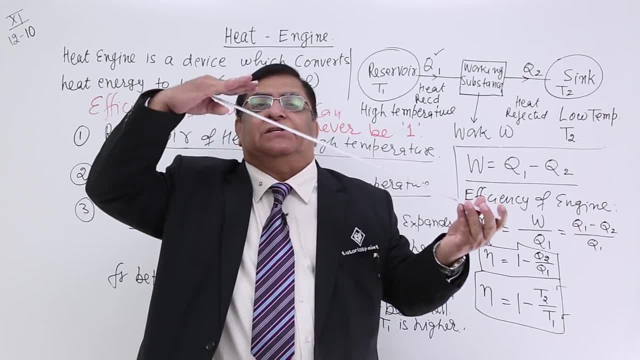 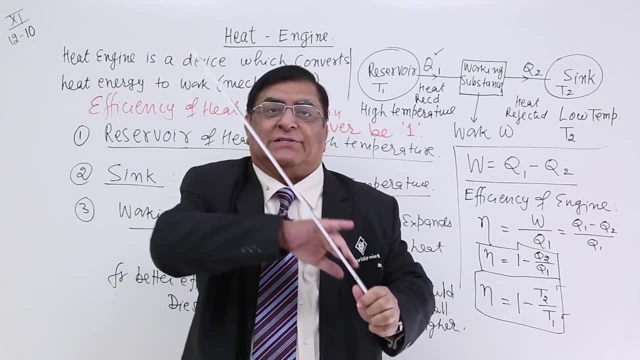 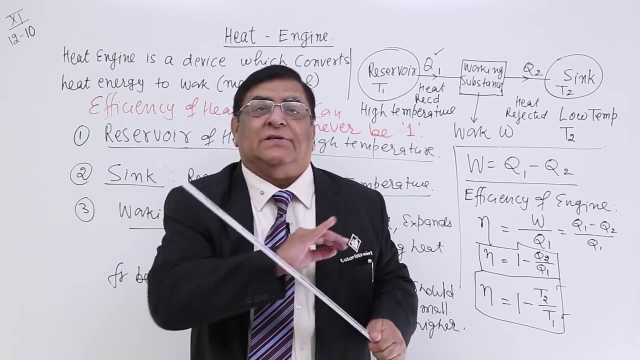 work. This is lower. engine is working, T1 is high, T2 is low, energy is flowing. If T2 is lower, oh, energy moves very fast. So lower, Lower is the atmospheric engine, more is the efficiency of the engine. 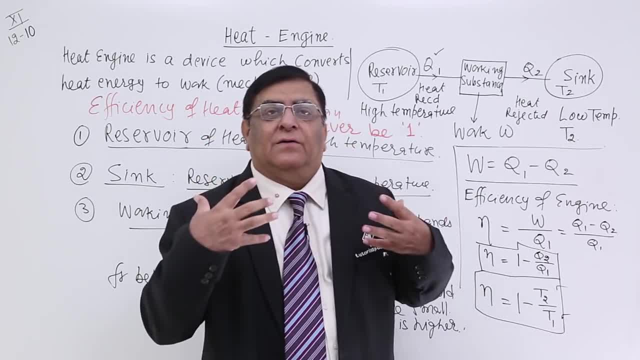 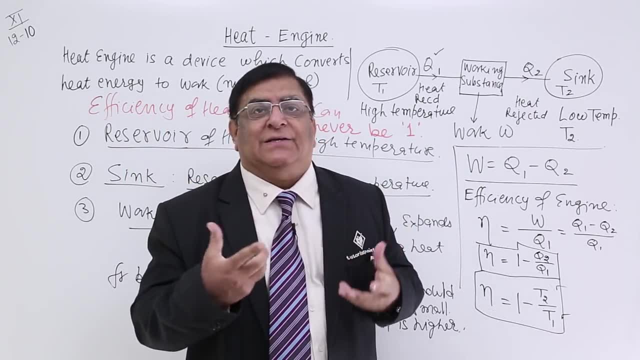 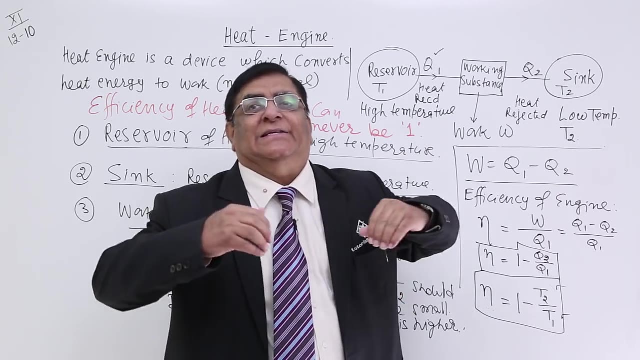 Human body is a heat engine. We are eating the food, converting it to burning it into heat, and that heat is converted by our body. our body is the working substance. we are doing work and heat is radiated out to sink. So this is the temperature of the air. this is the temperature of the air. this is the